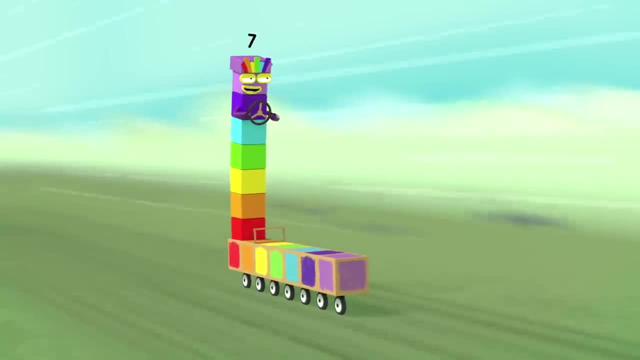 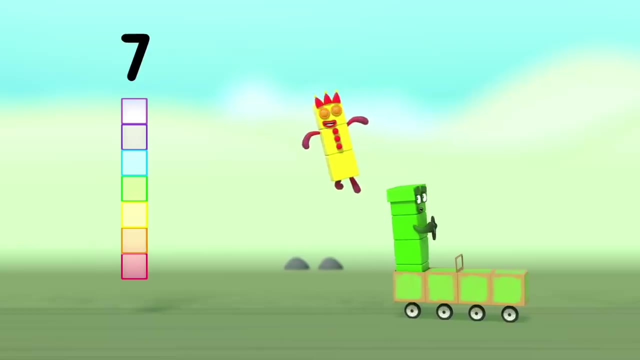 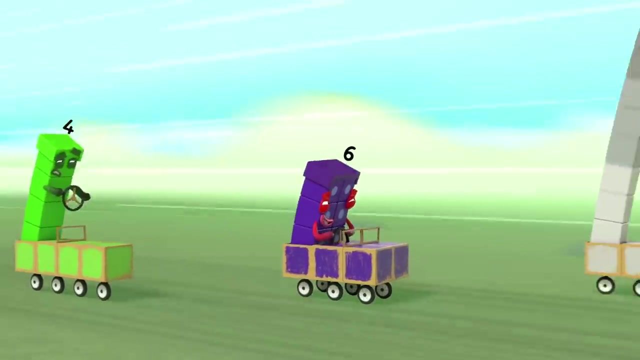 Look out, Phew, That was lucky. Whoo Whoa-ho-ho. 7 minus 3 equals 4! 4-wheel drive: Yay, Whoo, Yay, Whoo Yay. 6 has caught up with 9 as they enter the double dipper. 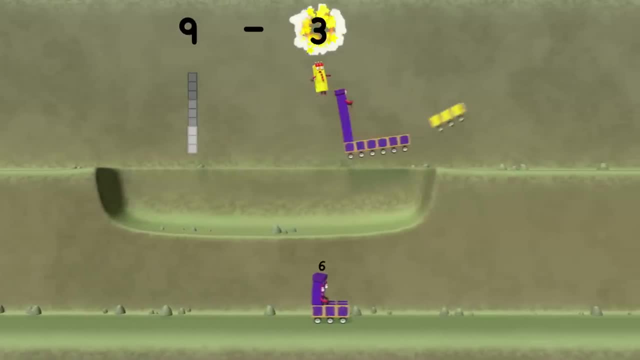 Mind that dip 9 minus 3 equals 6. And the double dipper takes 5 tips. liggerütter, bieber, sieb, And the double dipper takes 4 tips, And the double dipper takes 5 tips. 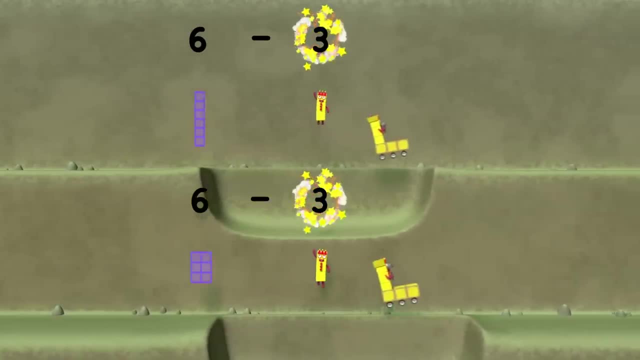 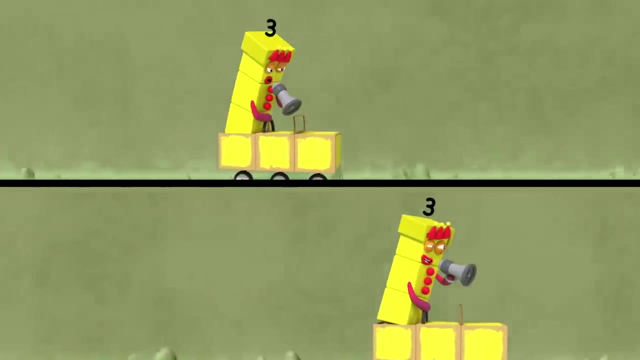 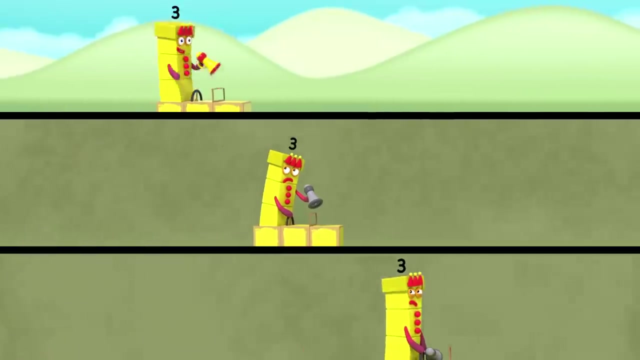 Double dicks. Six minus three equals three, And what a cloche for a nine. Six couldn't get fine there. Do you mind I'm commentating here? No, I'm commentating. No, I am Me, me, me. 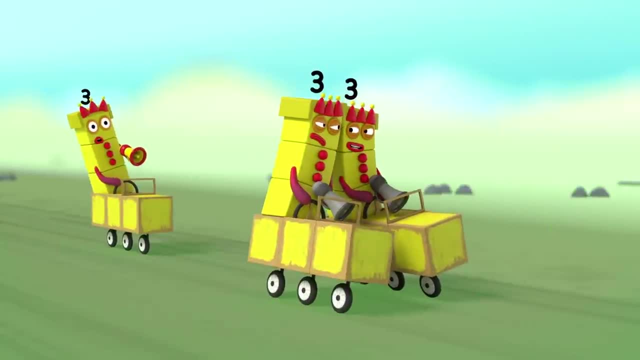 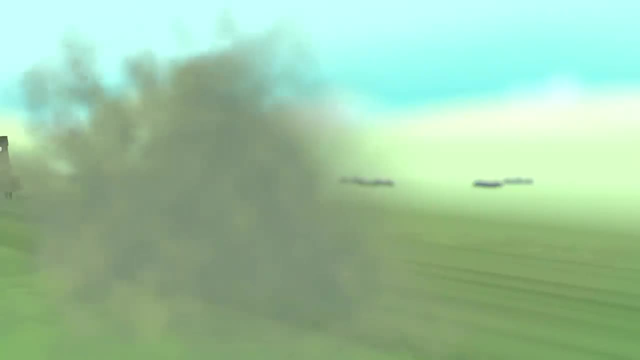 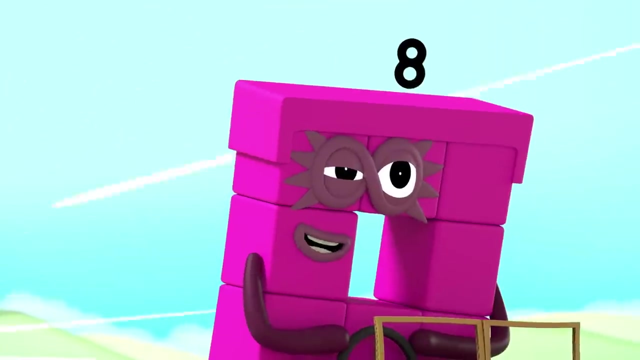 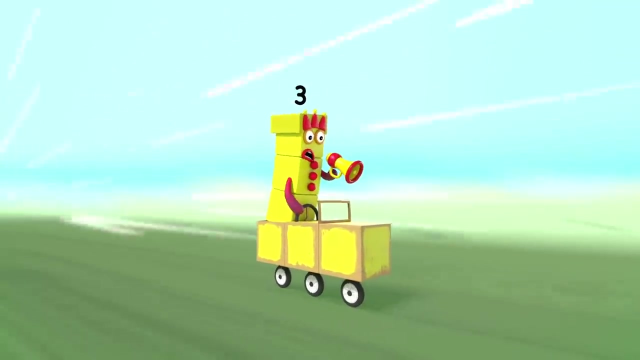 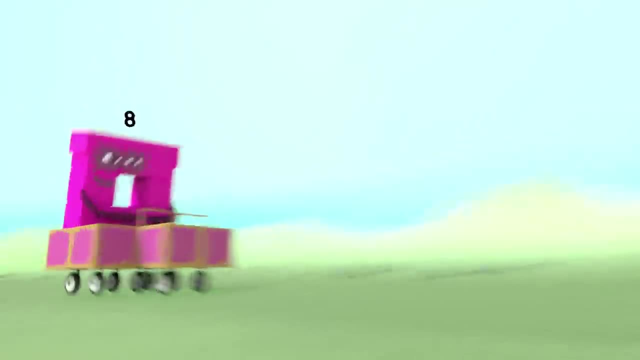 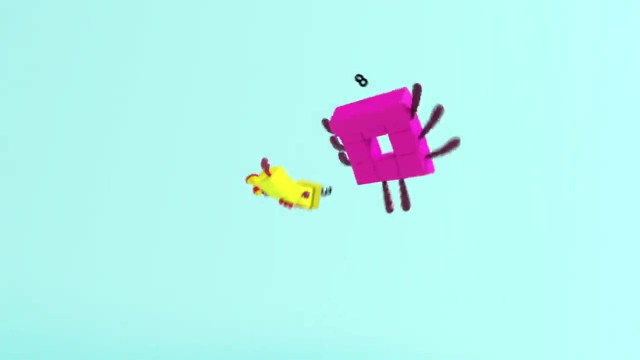 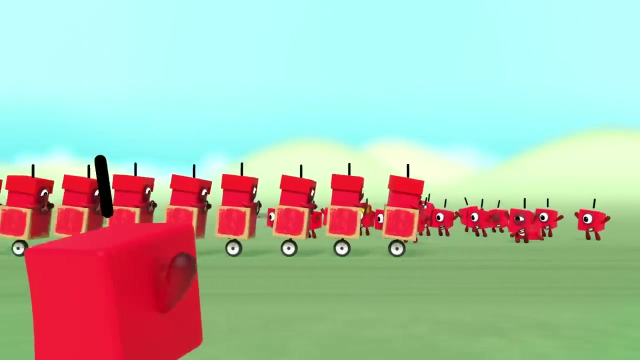 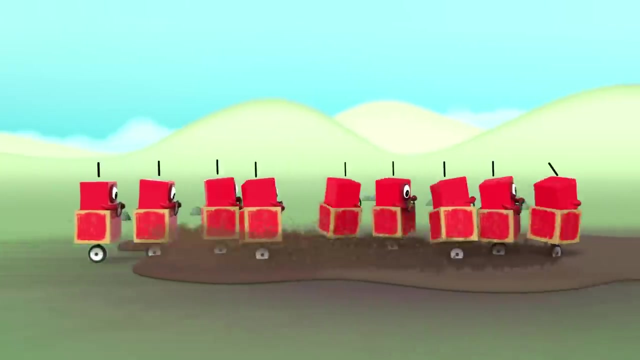 Octoblock coming through. Uh-oh, Uh-oh, Woo-hoo, Woo-hoo, Woo-hoo. And it's one in the lead, followed by one, but here's one coming up on the inside. Nine wolves equals. 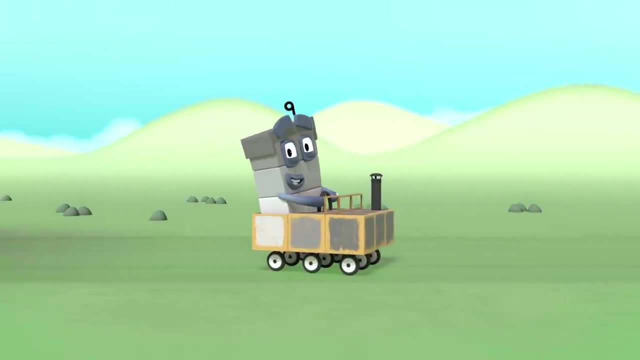 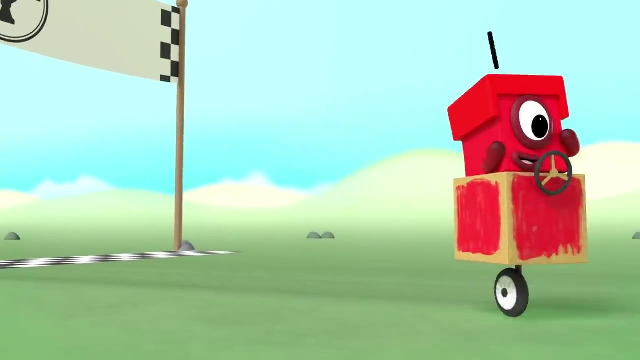 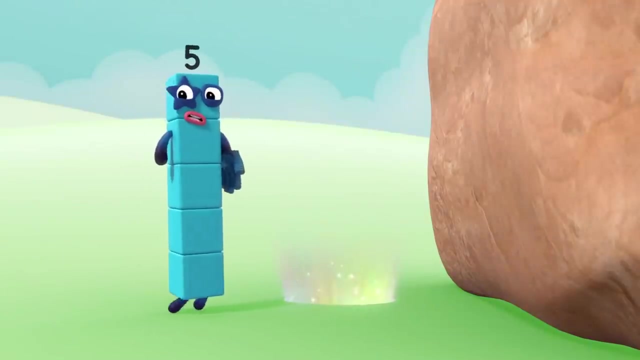 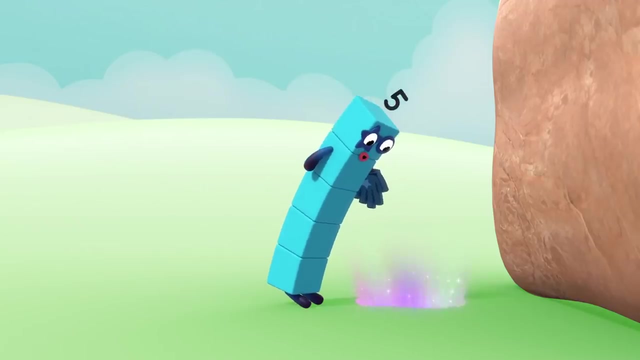 Nine, Nice day for it. I'm first. Oh yeah, Woo-hoo. What is that silly sucking sound? Oh, look a hole so big and wide. Why is it there? I do not know. I wonder what is down below. 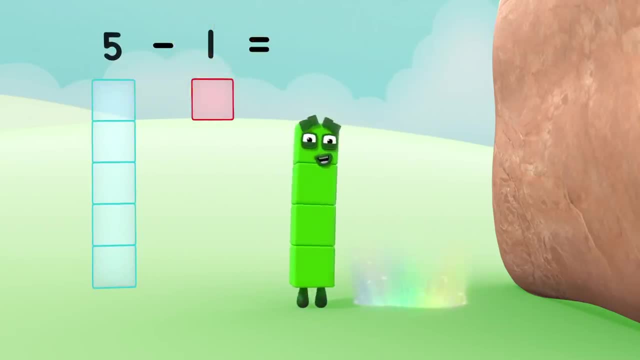 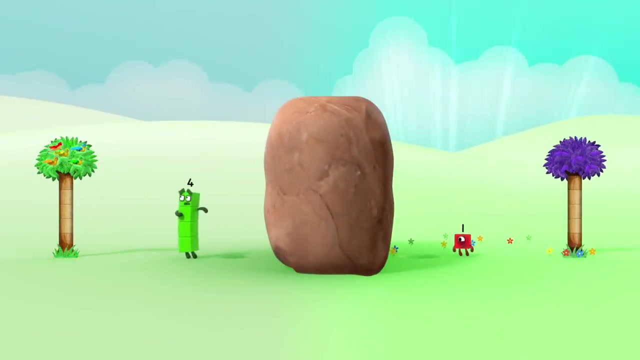 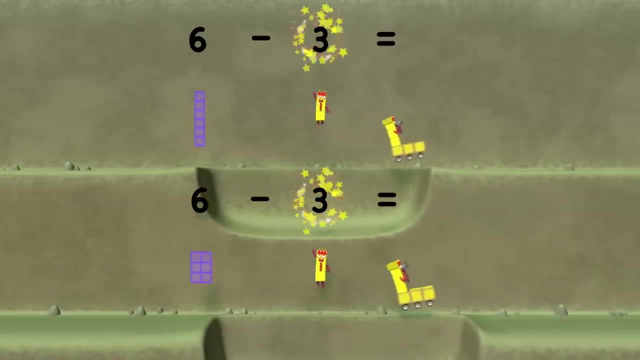 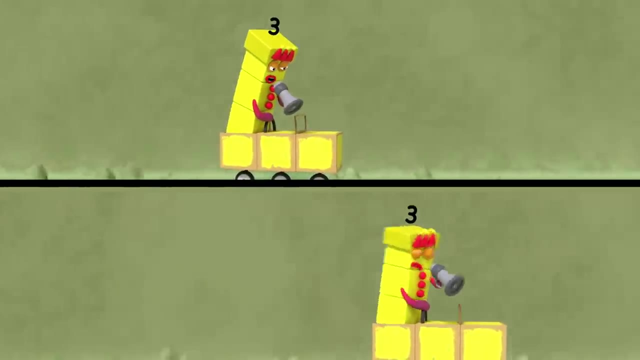 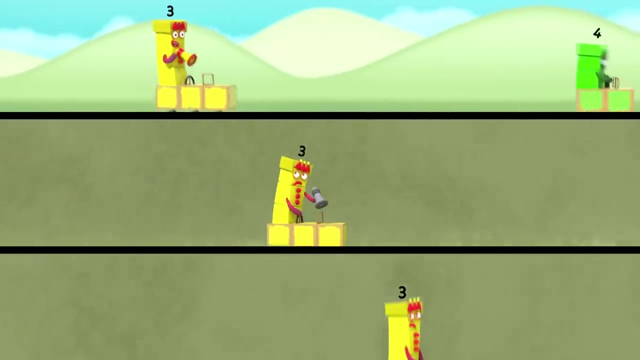 6 minus 3 equals 3.. And what a close shave for 9.. 6 couldn't get fine there. Do you mind? I'm commentating here? You, I'm commentating You, I am Me, me, me. 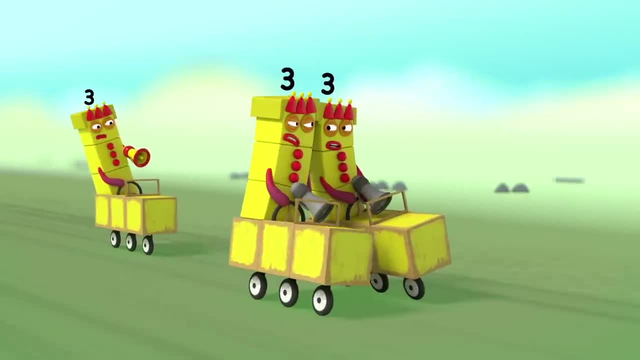 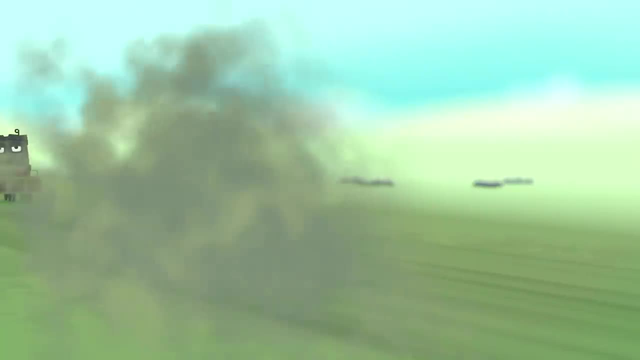 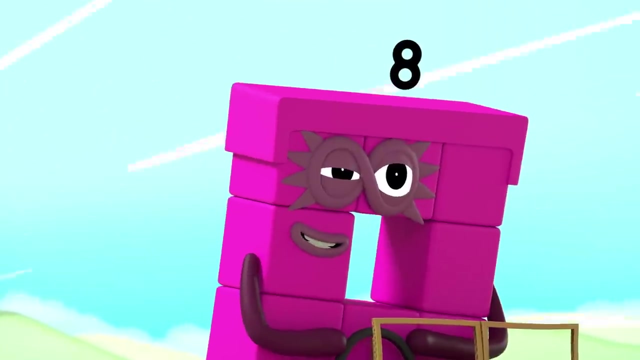 Me, me, me, You, Me, me, me. Pull yourselves together. 1, 3. 3. 3 equals me Achoo. Back in action And with the finish line in sight, It's 4 in the lead. 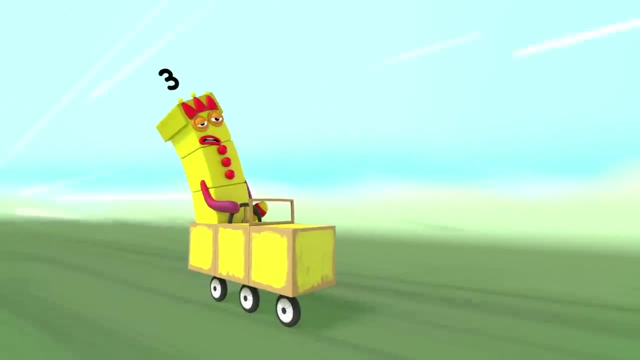 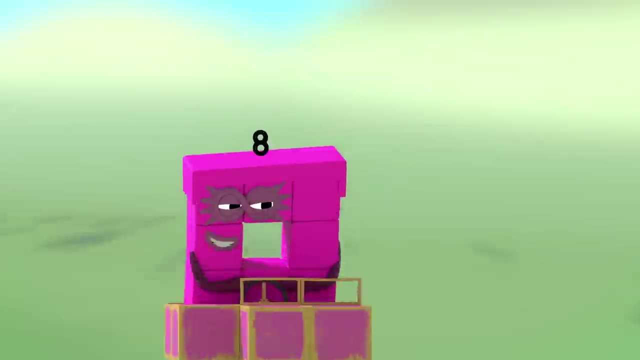 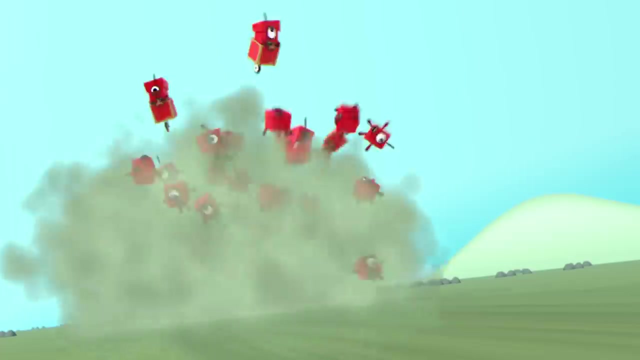 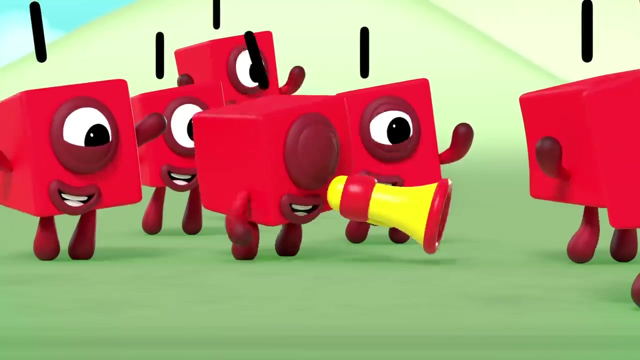 Then I need a breather Octoblock coming through. Uh-oh, Uh-oh, Ooh, Woo Woo, Woo, Woo Woo. And it's 1 in the lead, followed by 1.. But here's 1 coming up on the inside. 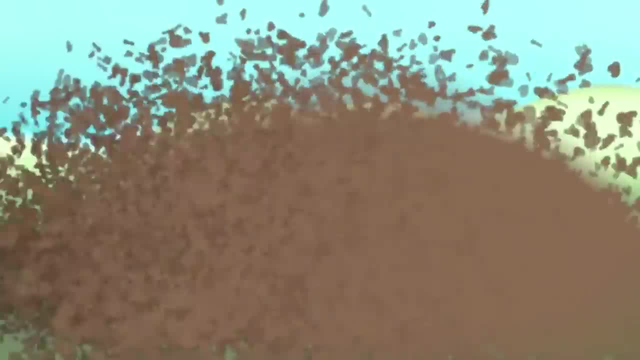 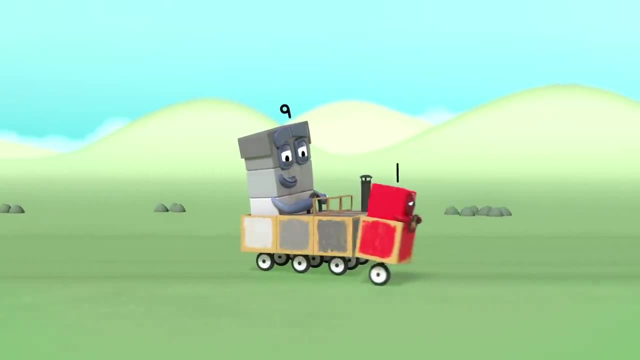 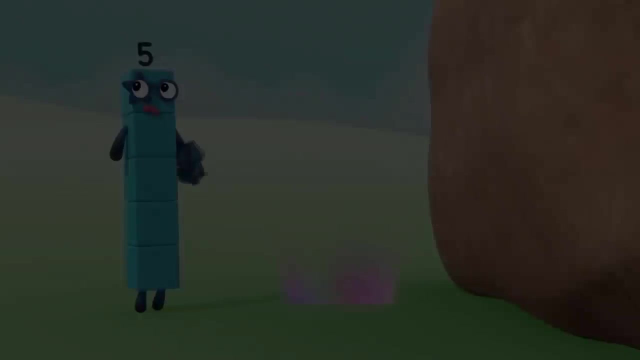 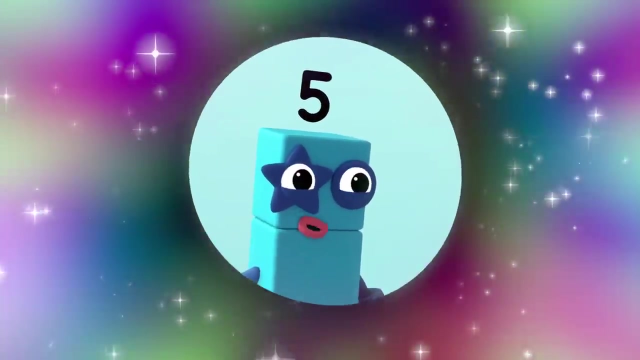 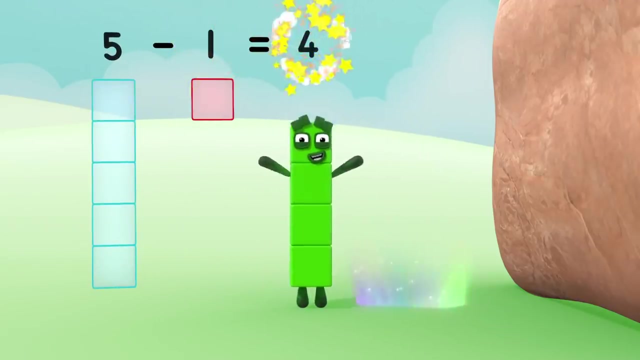 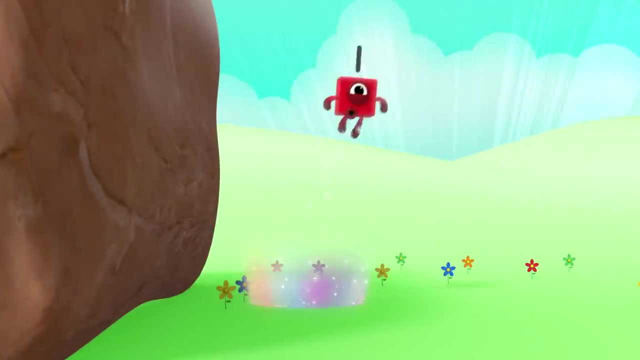 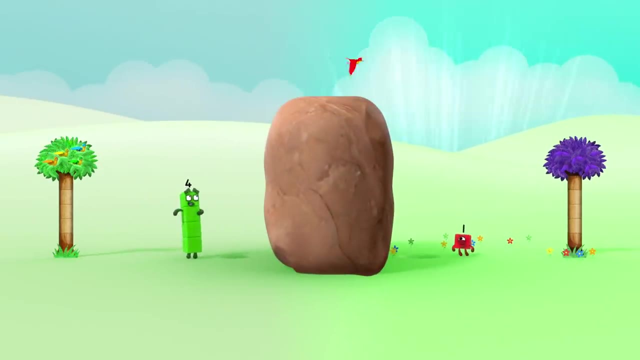 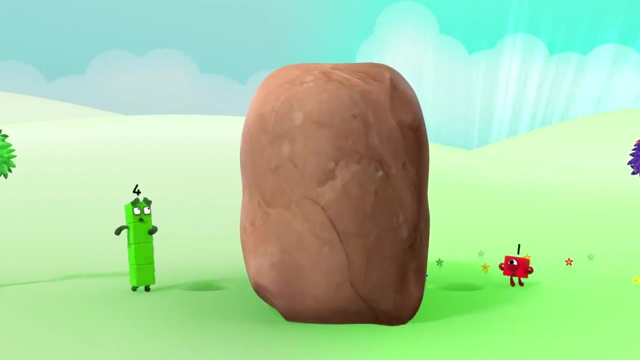 My head fell off. Where did it go? Woo-hoo, I have won. That was fun. Now I am four and here I am. I have won, Here I am. What a wonderful day to be alive. But where, oh, where, oh, where is five? 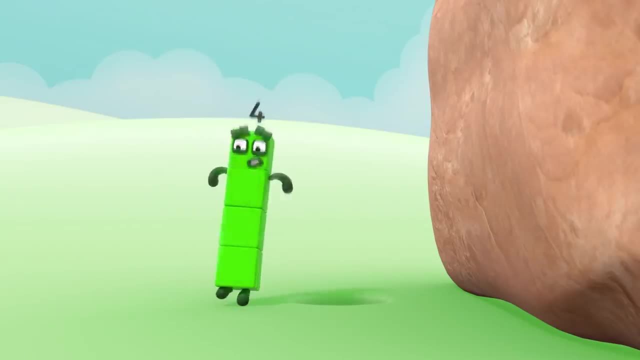 Five is gone. Where did she go? Is she all right? I do not know. Is she here? Is she there? I must keep looking everywhere. What is that silly sucking sound? A giant hole so big and round? Why is it there? I do not know. 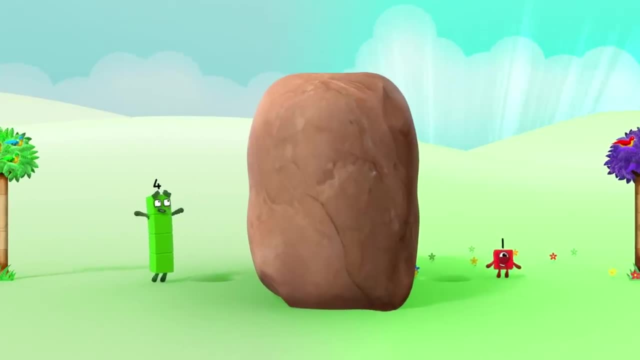 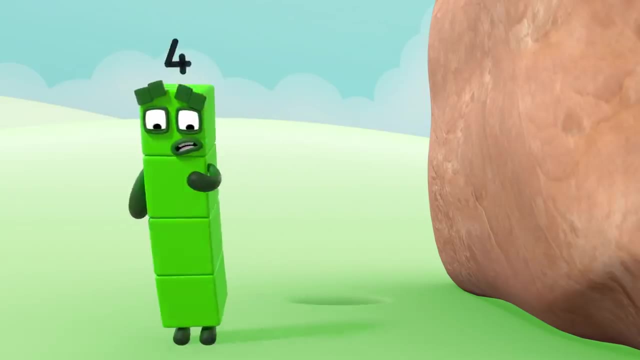 I am one Here. I am. What a wonderful day to be alive. But where, oh, where, oh, where, is Five? Five is gone. Where did she go? Is she all right? I do not know. Is she here? 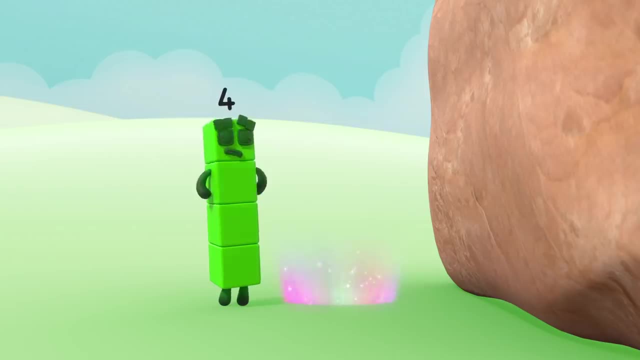 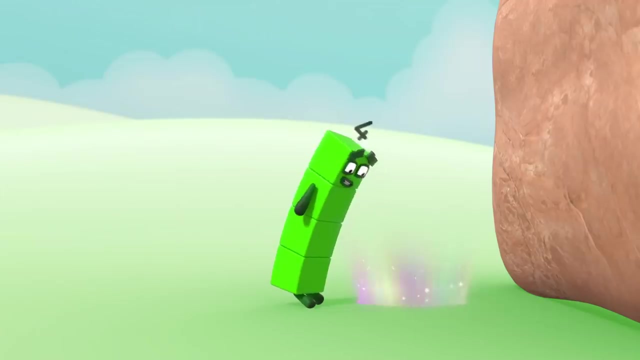 Is she there? I must keep looking everywhere. What is that silly sucking sound? A giant hole so big and round. Why is it there? I do not know. I wonder what is down below. Four Minus one Equals three. 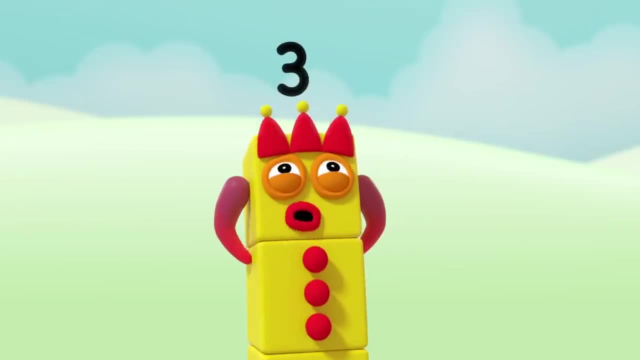 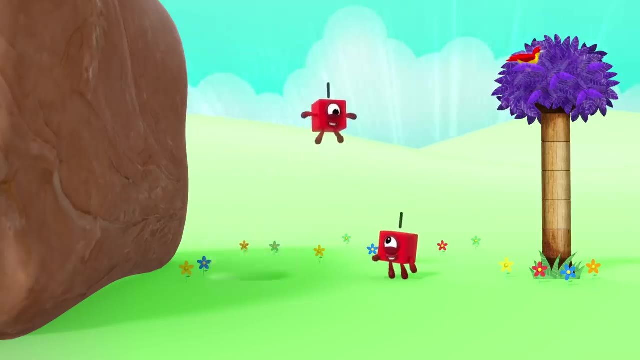 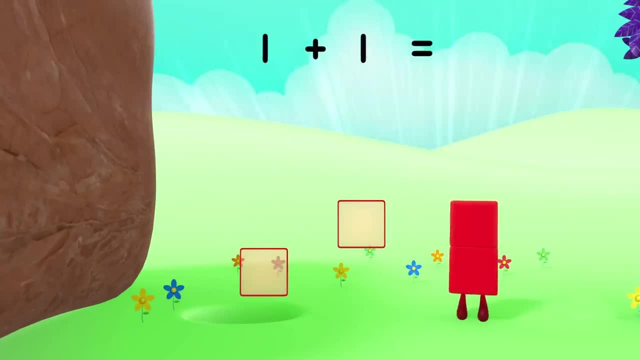 Did you see? Now I am three, and here I am. Now I am two and here I am. What a wonderful day to be alive. I wonder what is down below? Five minus one Equals four. Here I am. What a wonderful day to be alive. 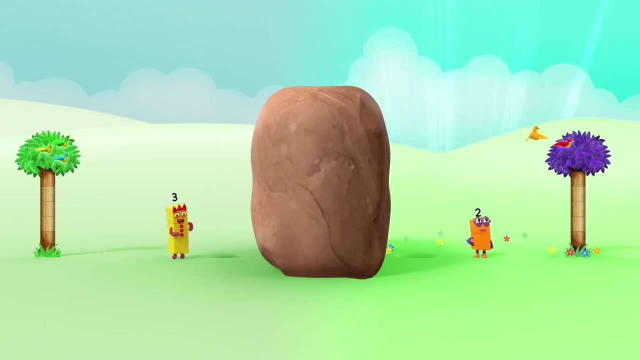 I am one, Here I am. What a wonderful day to be alive. Now I am four, and here I am. I am five, Here I am. What a wonderful day to be alive. But where, oh, where, oh, where is five? 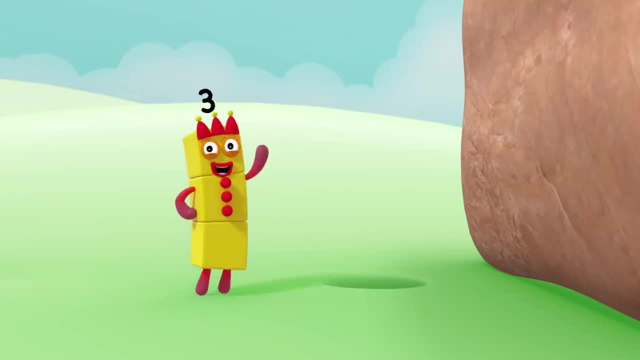 I was five, then four, then three. Someone has played a trick on me. I do not mind at all. you see, Three is who I want to be. What is that silly sucking sound? A giant hole so big and round. 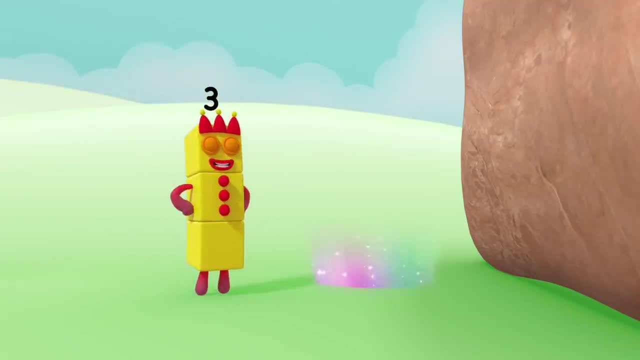 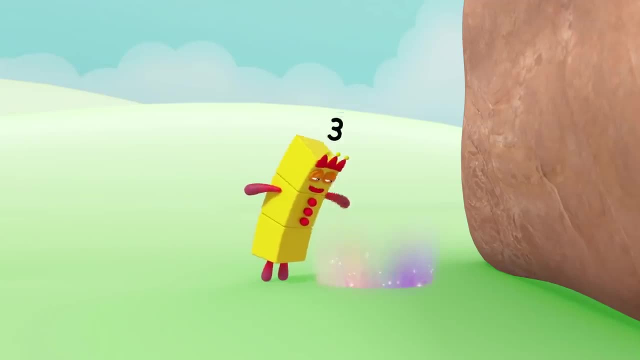 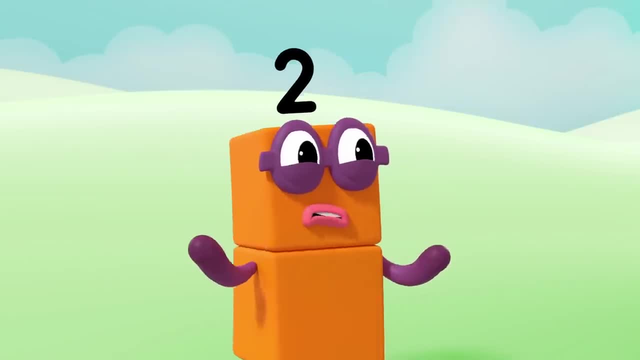 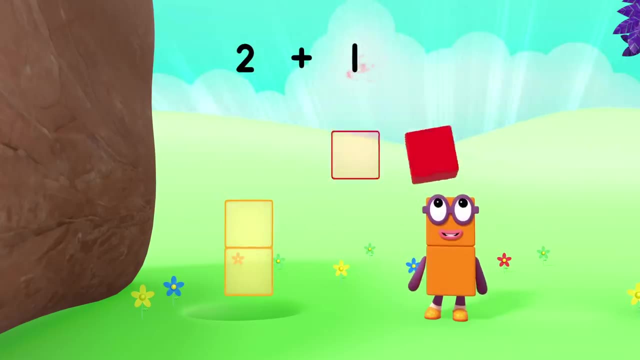 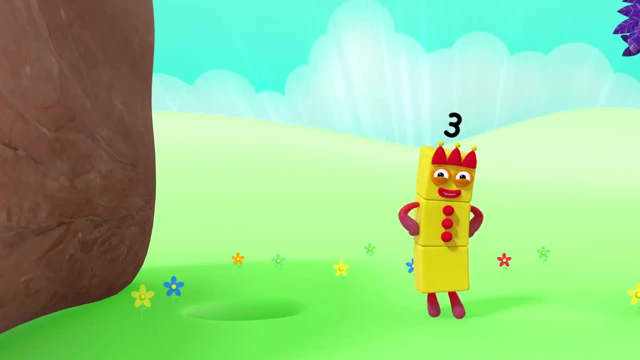 Did you see? Now I am two and here I am. Now I am three and here I am. What a wonderful day to be alive. But where, oh, where, oh, where is five? I wonder where the world is. 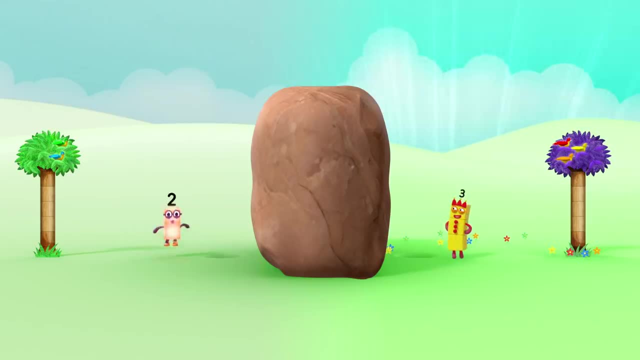 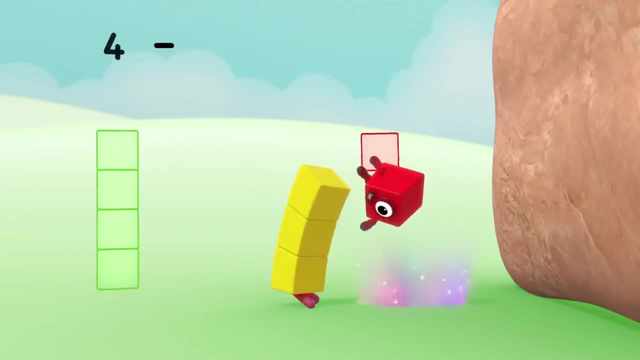 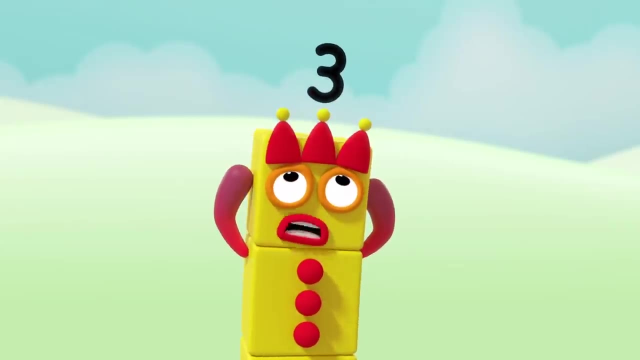 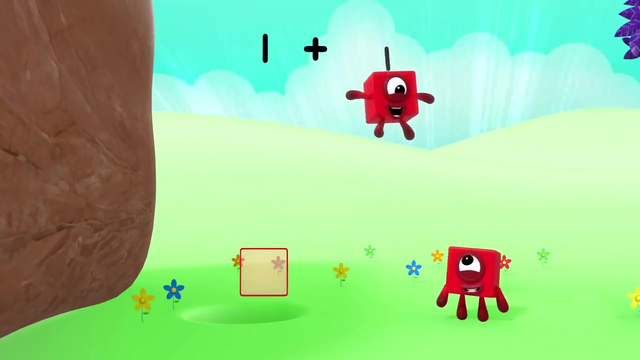 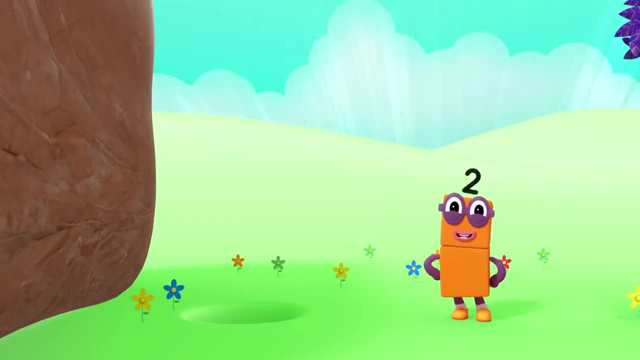 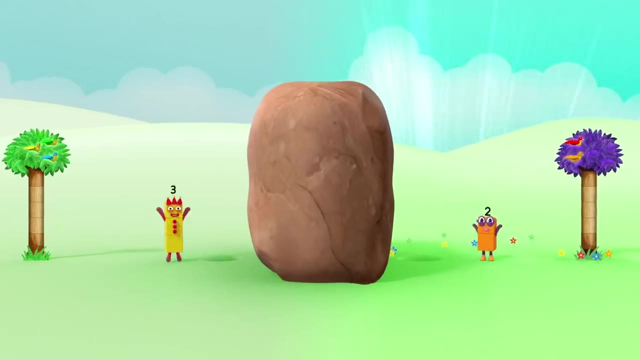 What is happening to me? I just got bigger, Did you see? Now I am three and here I am. Now I am two and here I am. What a wonderful day to be alive. But where, oh, where, oh, where is five? 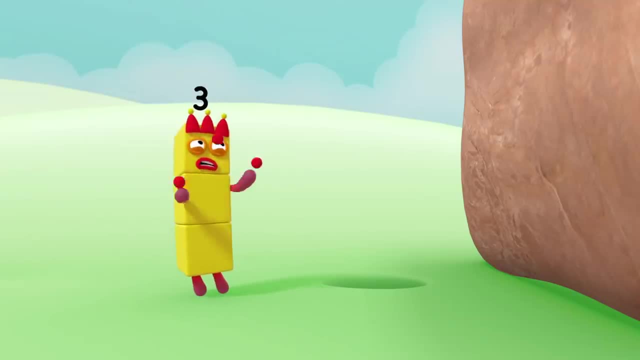 I was five and four and three. Someone has played a trick on me. I do not mind at all. you see, Three is who I want to be. What is that silly sucking sound? A giant hole so big and round. Why is it there? I do not know. 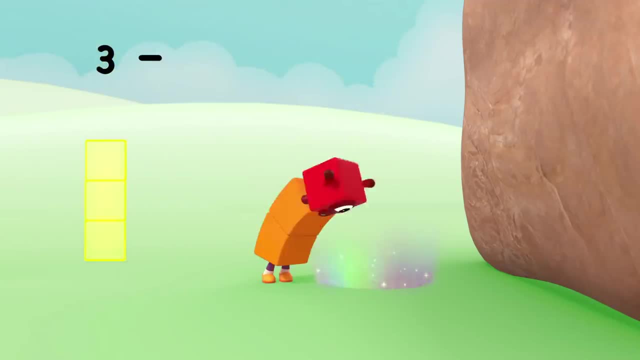 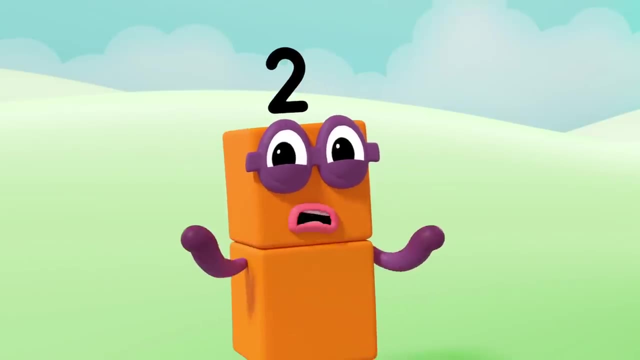 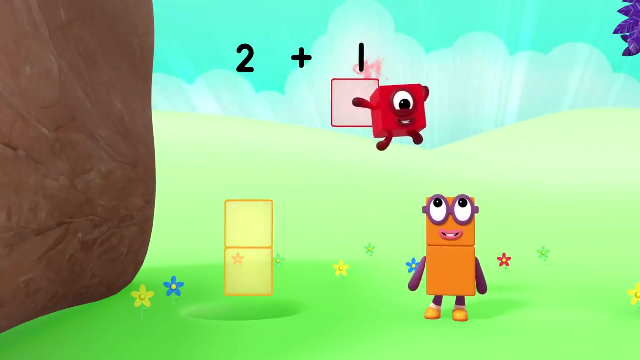 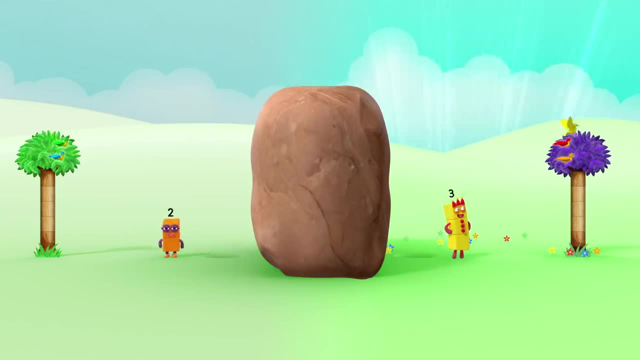 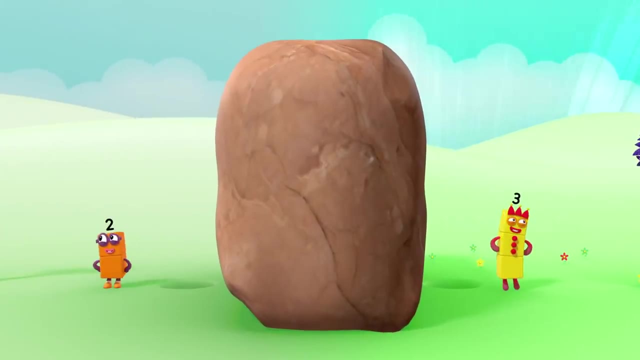 What is happening to me? I just got bigger, Did you see? Now I am two and here I am. Now I am three and here I am. What a wonderful day to be alive. But where, oh, where, oh, where is five? 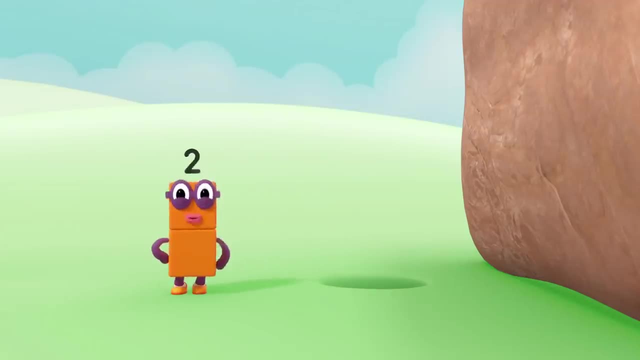 I wonder where the ones will go. I think I've got it Now. I know Every time we get one smaller, somewhere else is getting taller. What is that silly sucking sound? A giant hole so big and round? Why is it there? I do not know. 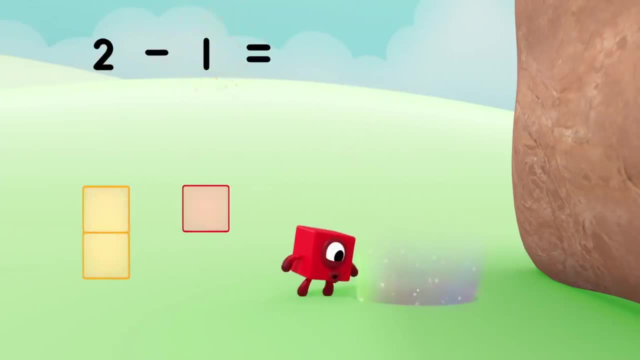 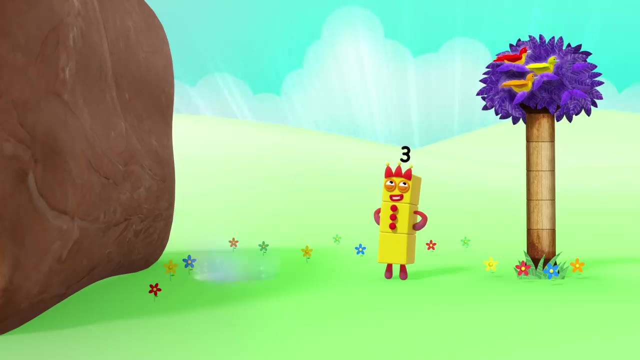 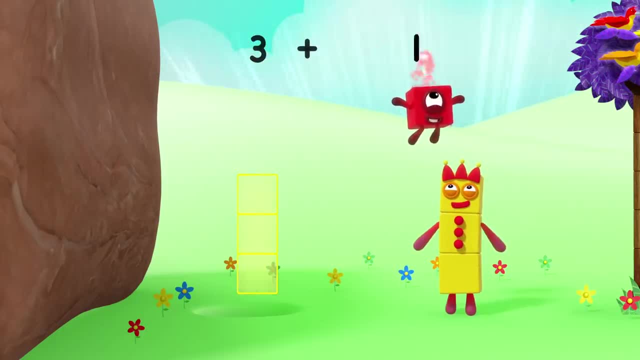 What is happening to me? I just got bigger, Did you see? I am one. That was fun. Three plus one equals four. What is happening to me? I just got bigger, Did you see? Now I am one, and here I am. 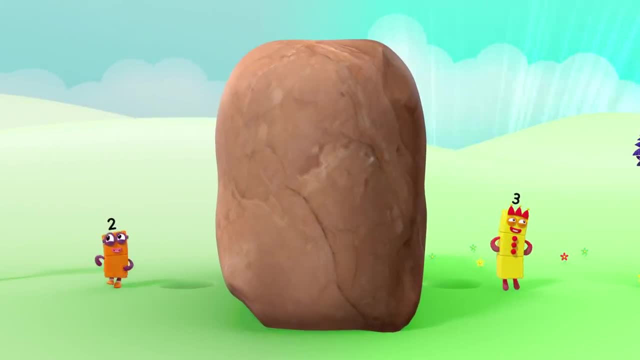 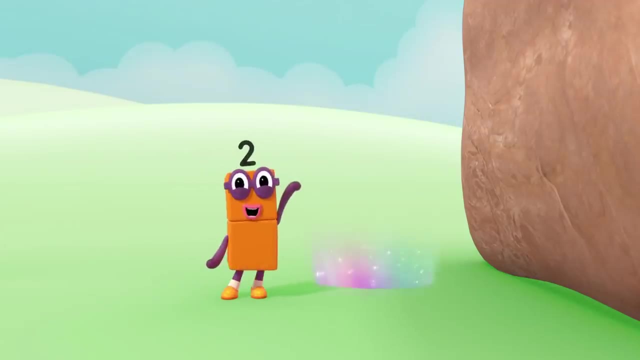 My head fell off. Where did it go? I am one. That was fun. Two And three. I am two Minus one Equals three. Whoa, I am three. No, I am one Minus three. 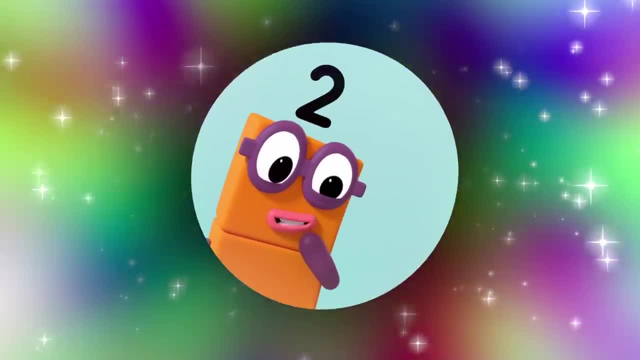 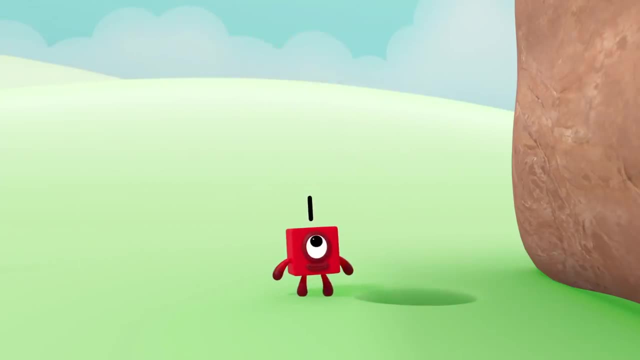 I am two Minus Minus one. He visited Earth. Cool See, we are so much faster Now. there is two. I can make it yesterday. No, I will make it tomorrow, But no, You can't do this now. 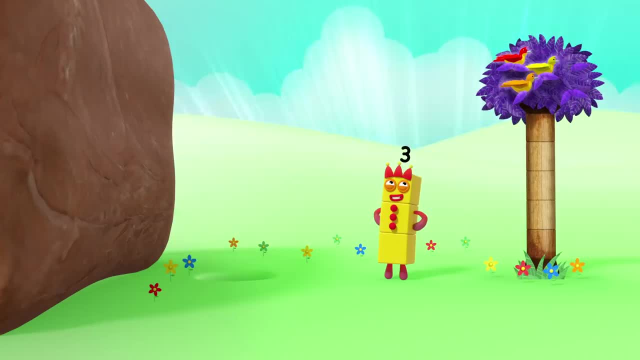 I win this Example Two to Study Culture: Scary and exciting. Ahhh, that's great. I'm so happy. It's a nice idea. I got wandering week. I still have four on the train, I can do it, YAY. 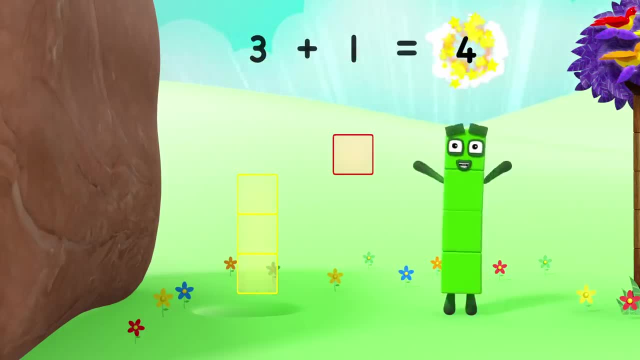 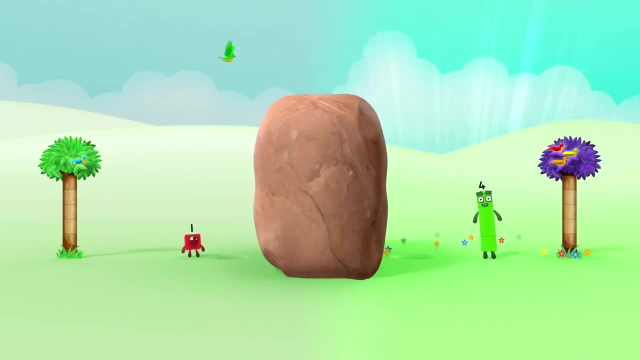 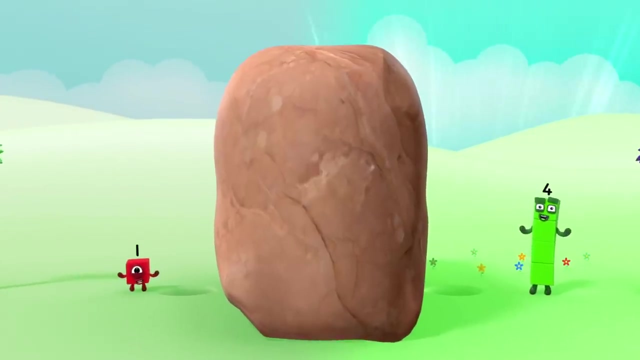 Yay, Three plus one equals four. What is happening to me? I just got bigger, did you see? Now I am one and here I am. Now I am four and here I am. What a wonderful day to be alive. But where, oh, where, oh, where, is five? 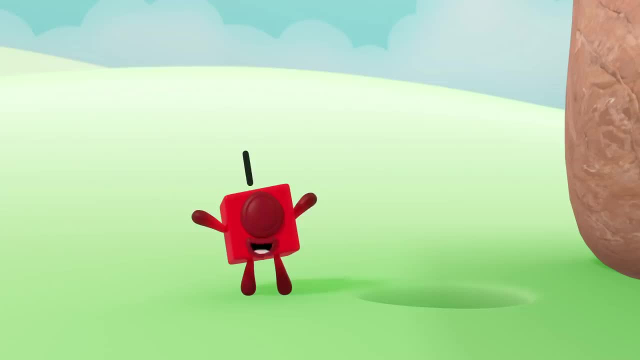 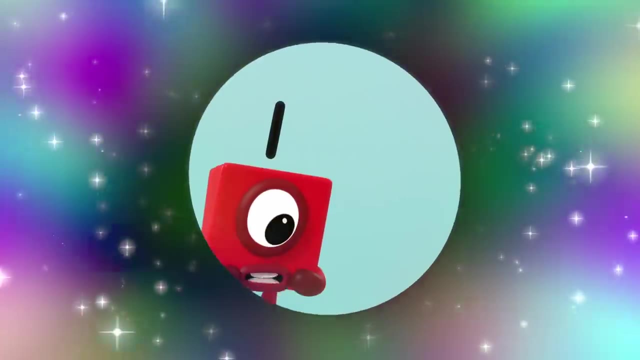 Five, four, three, two, one. Someone's having lots of fun. Now I know where five will be. Four is waiting there for me. What is that silly sucking sound? A giant hole so big and round. Why is it there? I think I know. I think I know what's down below. 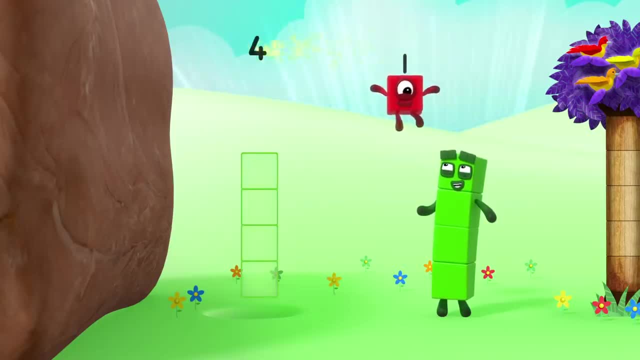 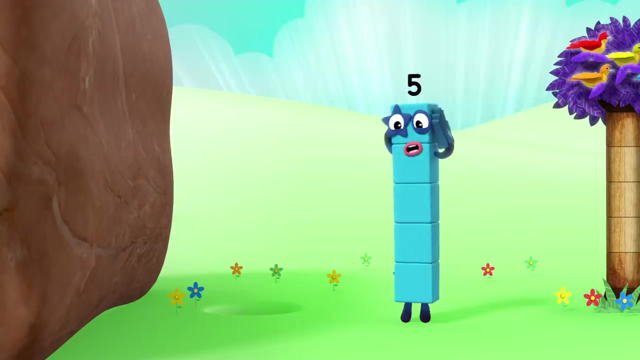 I am one. That was fun. Four plus one equals five. What is happening to me? I just got bigger. did you see? What a wonderful day to be alive. But where, oh, where, oh, where is five? Here I am. 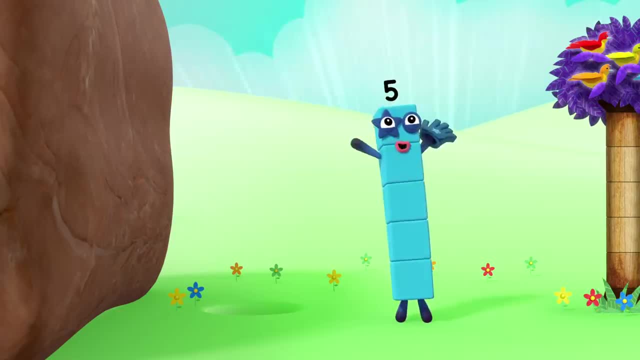 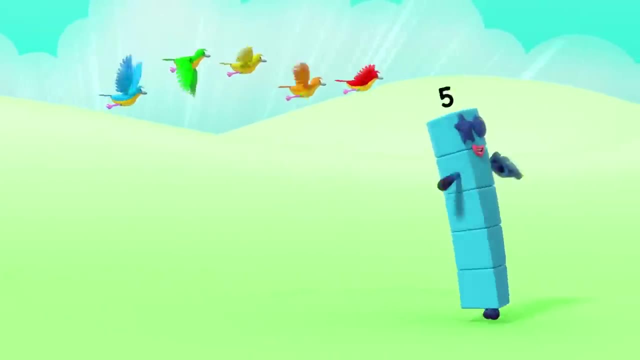 I am and I am five. What a wonderful way to arrive. One, two, three, four, five. What a brilliant, amazing, fantastic, terrific and wonderful day to be alive. One, two, three, four, five. Hello, We're playing hide and seek. 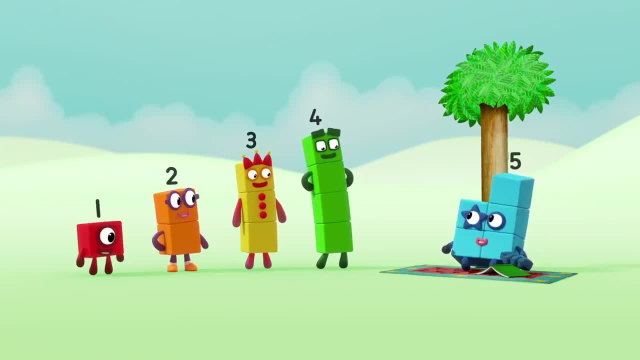 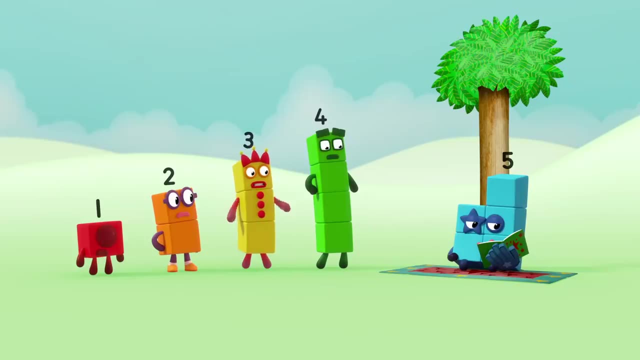 Want to join in. I would absolutely love to You hide, And I'll see, And I'll see. You won't find us sat there. Oh, will I not? now? I'm good at this game. I'll find you and point you out. 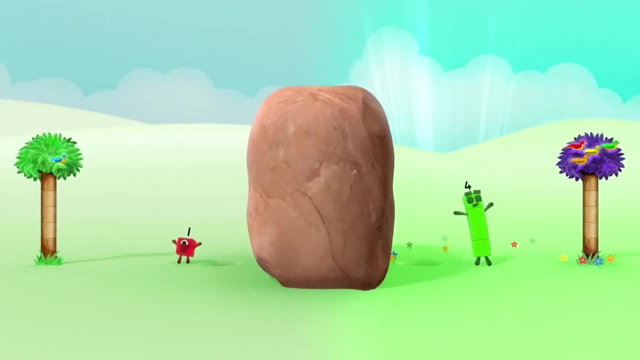 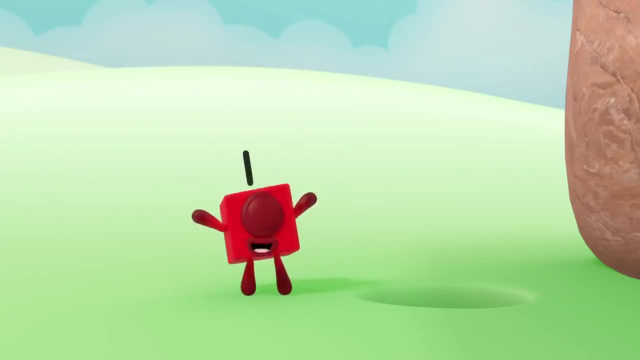 Now I am four and here I am. What a wonderful day to be alive. But where, oh where, oh, where, is five? Five, four, three, two, one. Someone's having lots of fun. Now I know where five will be. 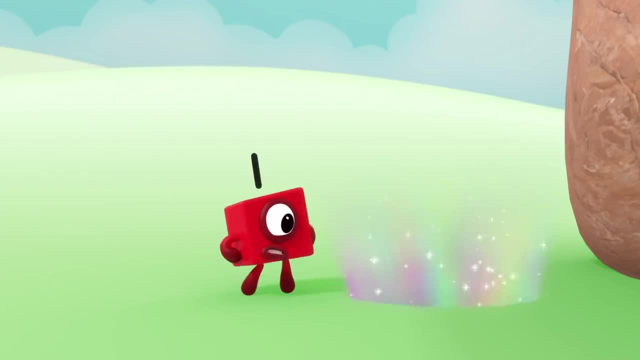 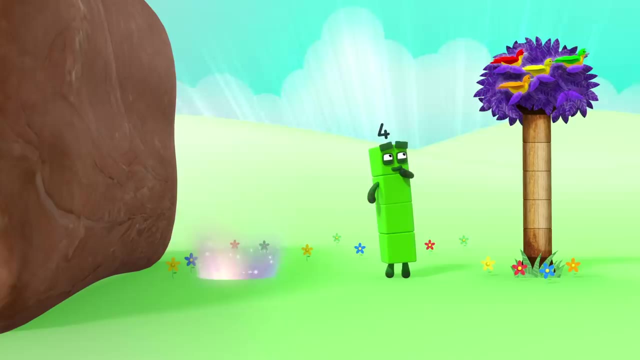 Four is waiting there for me. What is that silly sucking sound? A giant hole so big and round? Why is it there? I think I know. I think I know what's down below. I am one. That was fun. Four: 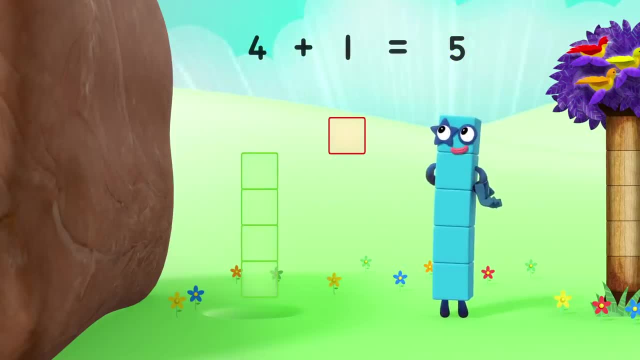 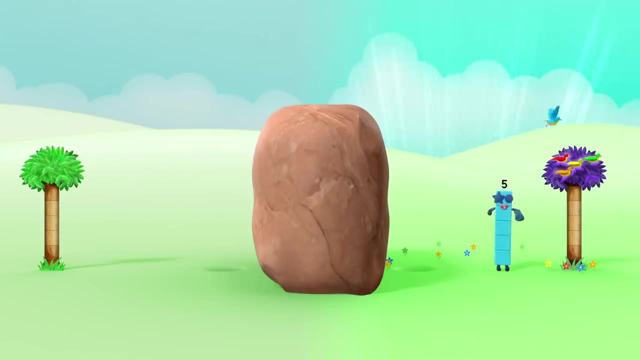 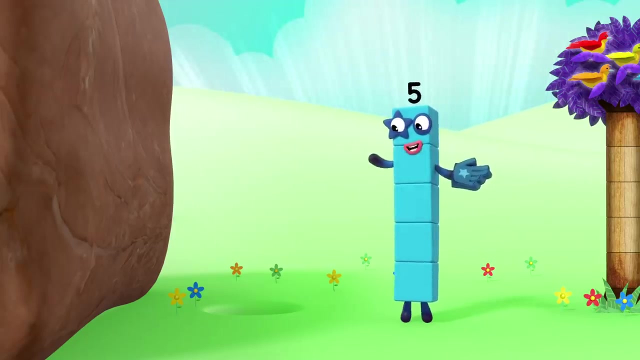 Three plus one equals five. Three plus one equals five. What is happening to me? I just got bigger. Did you see? What a wonderful day to be alive. But where, oh, where, oh, where is five? Here I am and I am five. 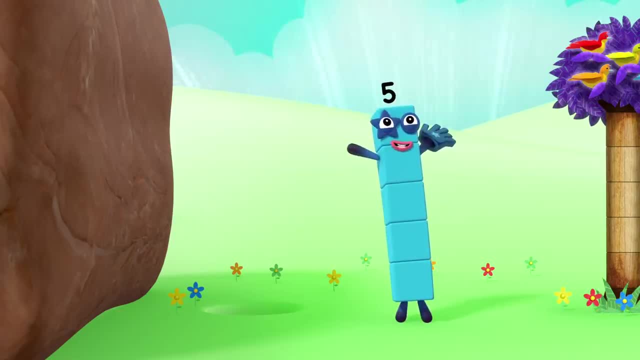 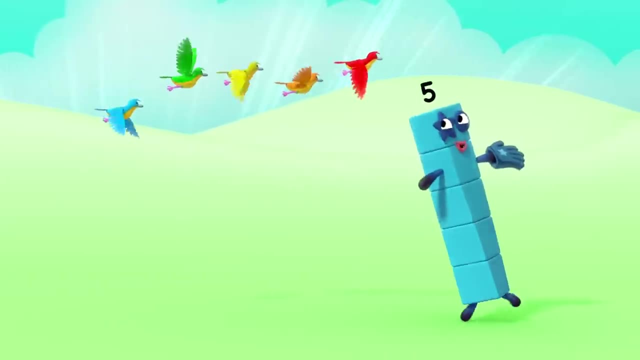 Here I am and I am five. What a wonderful way to arrive. What a wonderful way to arrive: One, two, three, four, five. What a brilliant, amazing, fantastic, terrific and wonderful day to be alive: One, two, three, four, five. 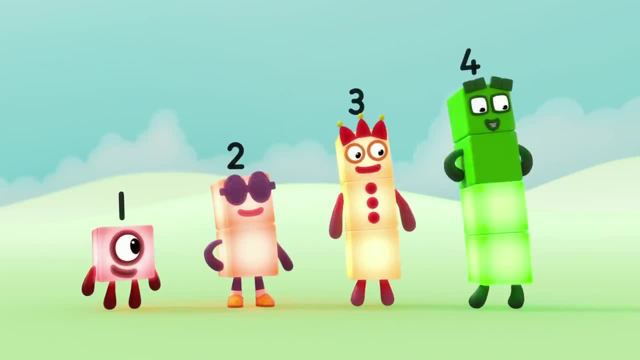 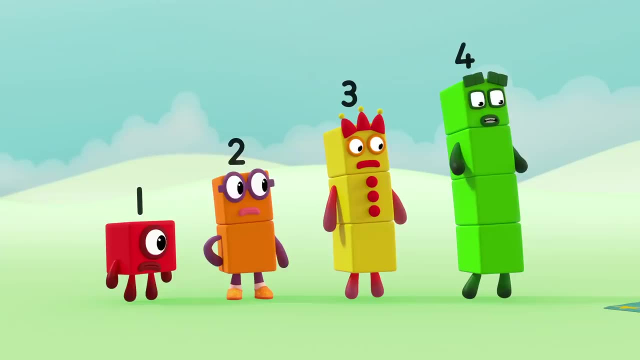 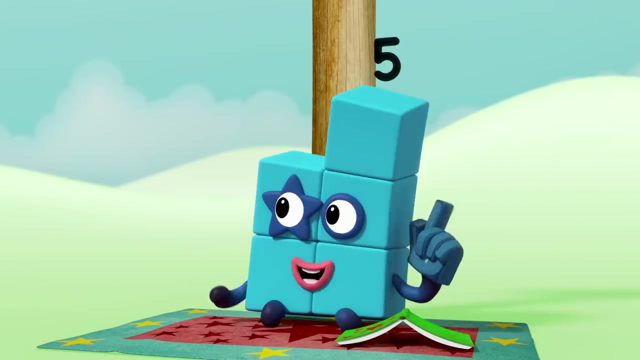 Hello, We're playing hide and seek, Want to join in. I would absolutely love to You hide and I'll seek. You won't find us sat there, Oh, will I not? now I'm good at this game. I'll find you and point you out. 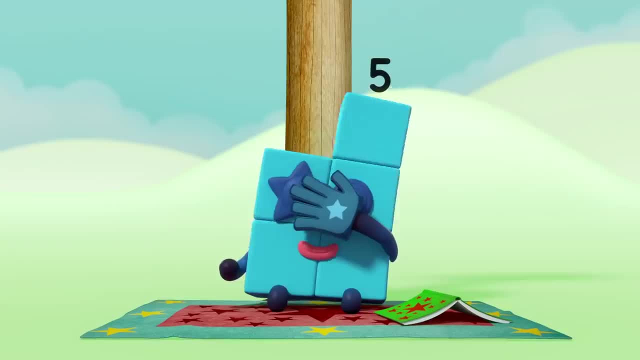 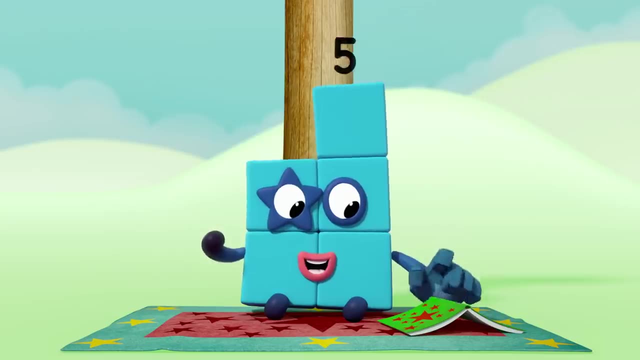 One, two, three, four five. One, two, three, four five. One, two, three, four, five. Ready or not here I? Ready or not here I Get on with my book. Get on with my book. 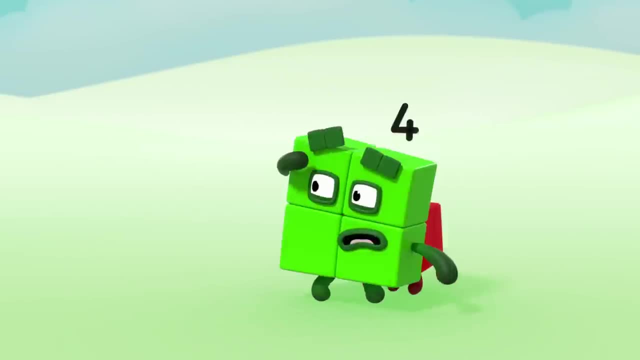 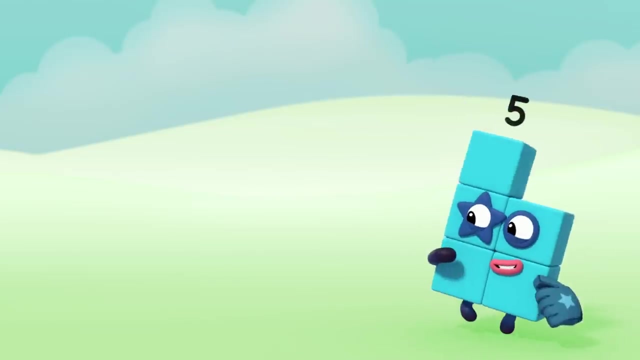 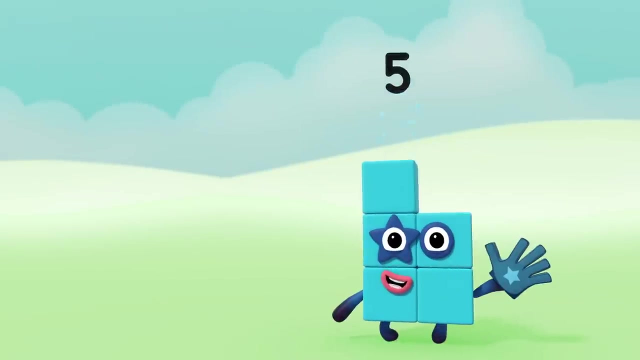 Hey, hide behind me. Hey, hide behind me. Where can I hide? I know behind you Four, Oops, Four Plus one equals five. Ready or not, here I come. Find you four, Find you one. Five minus one. 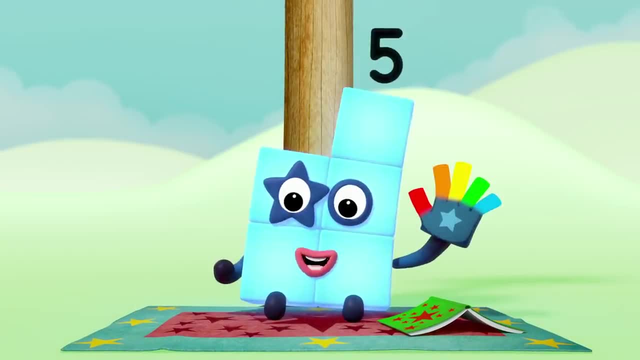 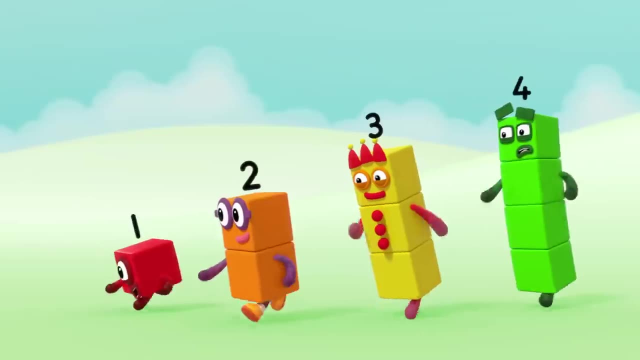 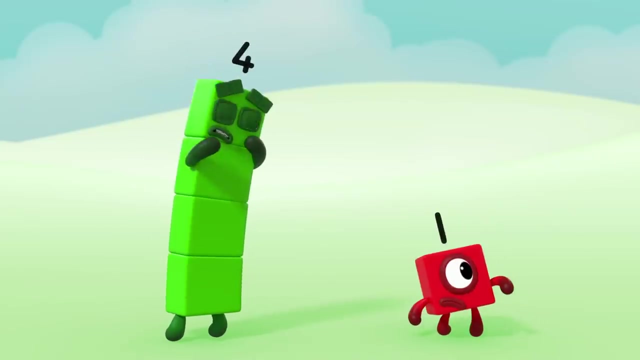 One, two, three, four, five, Ready or not, here I Get on with my book. Oh my God, You put someone out, Nailed it. Respect, Are you saying your? Now please let me in. 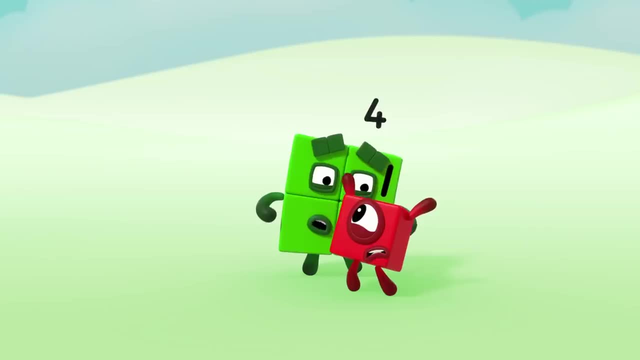 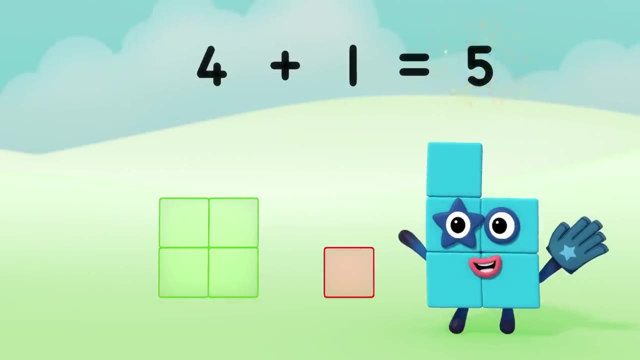 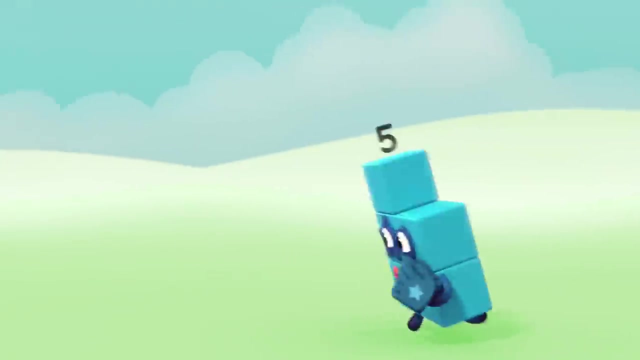 Now, please, the two of you, and find somebody who is better to you. Sorry, Ah Hey, Hide behind me. Where can I hide? I know behind you. Four, Oops, Four Plus one Plus one Half. 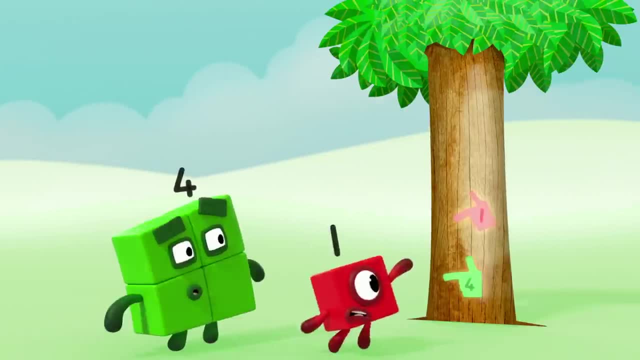 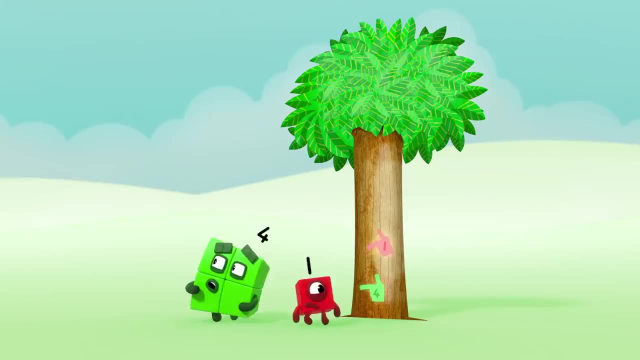 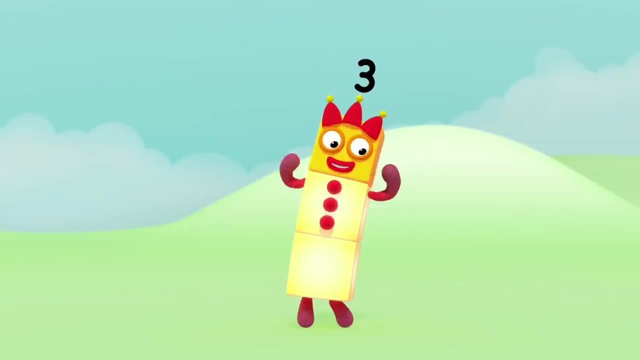 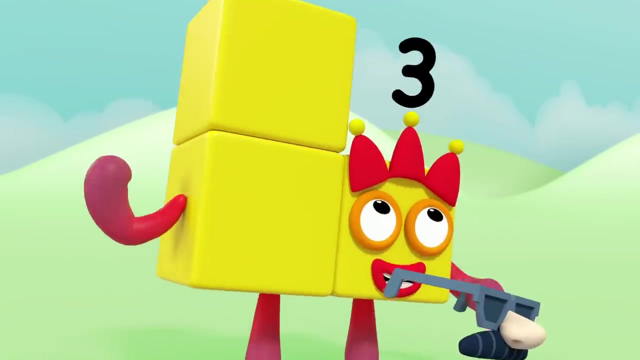 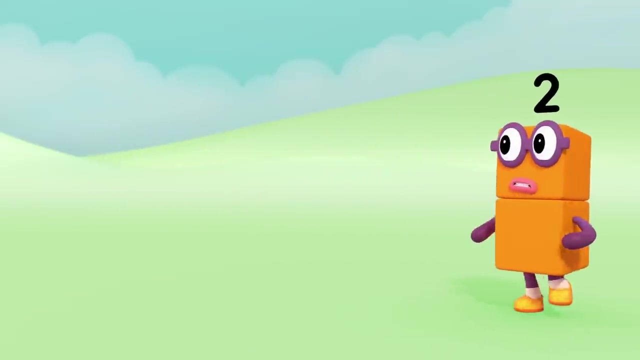 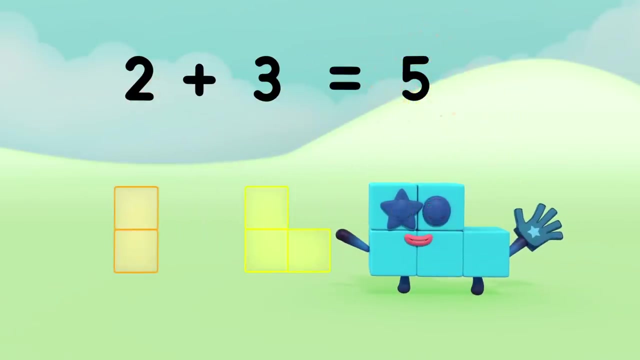 Look Five, said she'd point us out. Five was right here. How I am. Three Master of Disguise. Ah, Shhh, Shhh, Shhh. Two Plus three Equals Five. Ready or not, here I be. 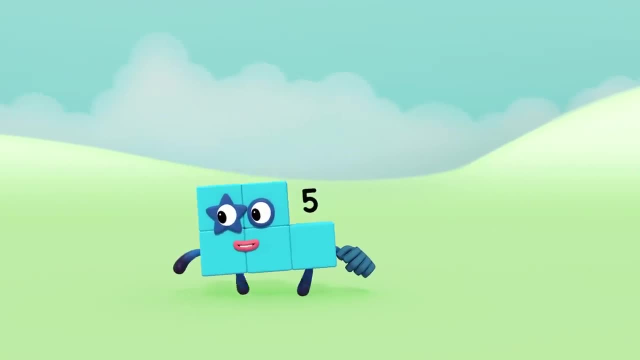 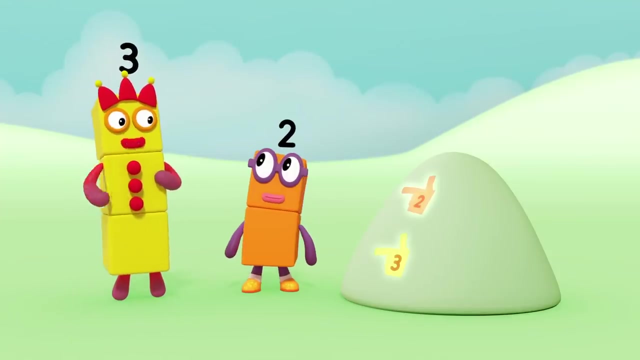 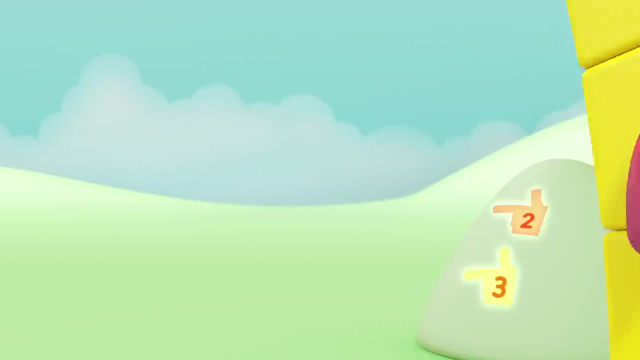 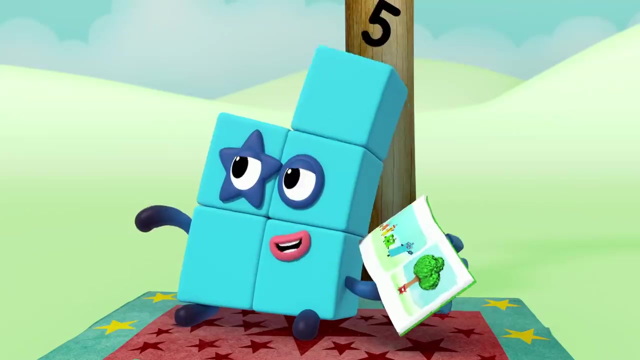 Find you two, Find you three. Five minus three Equals two. A pair of pointing prints. Five found us. But but how? Eh Five You're here. How did you Told you I was good? Now my turn to hide. 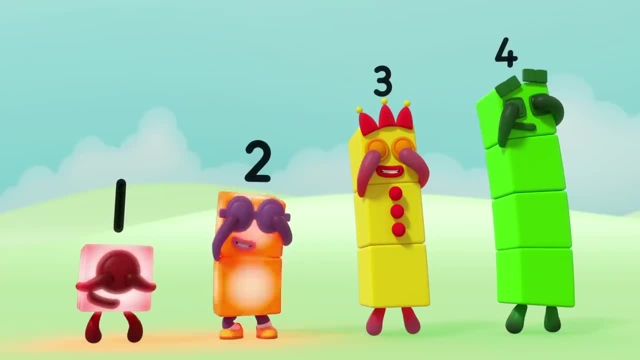 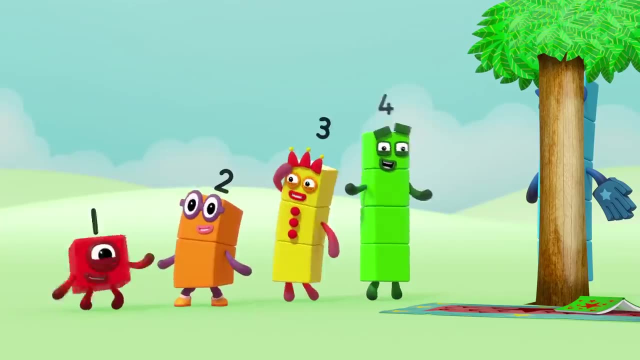 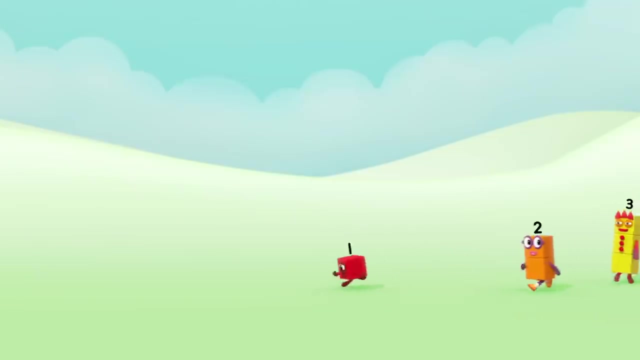 On we go. One, Two, Three, Four. Ready or not, Five here we come. Ah Ooh, You're nothing but a cheetah Rock. One Plus four Equals Five. Found you A-me-zing. 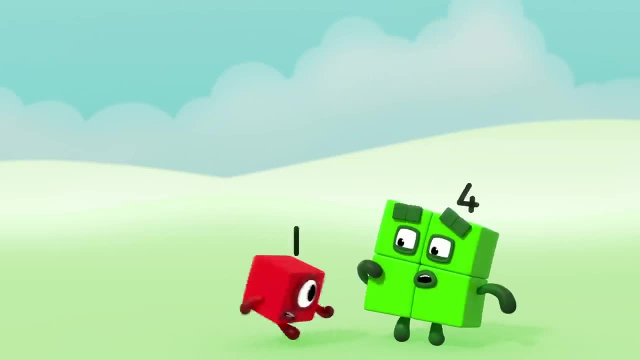 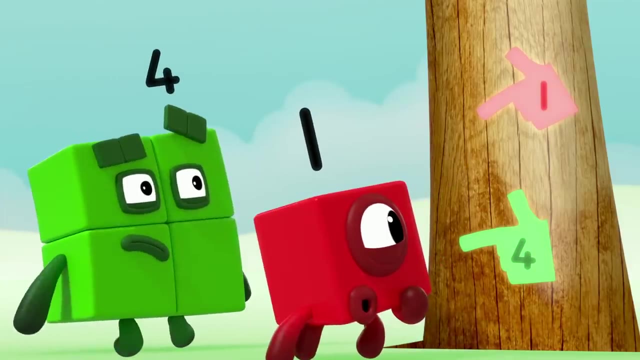 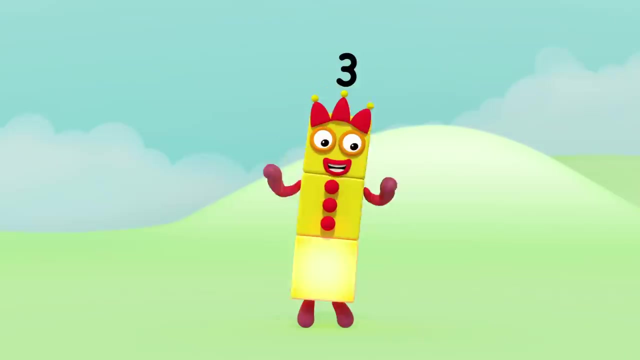 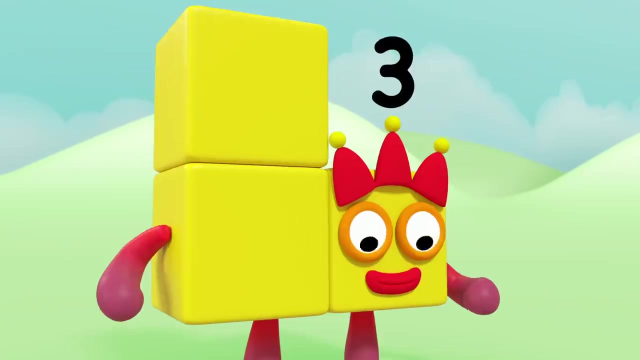 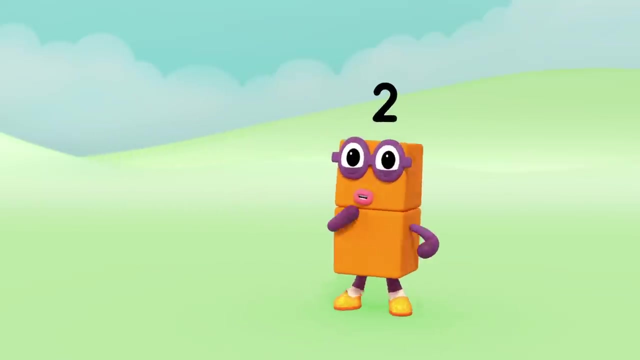 Equals four. Look Five, said she'd point us out. Five was right here. How I am three Master of disguise. I am three, Master of disguise. Master of disguise, Ah, Shh, Uh, Shh Two. 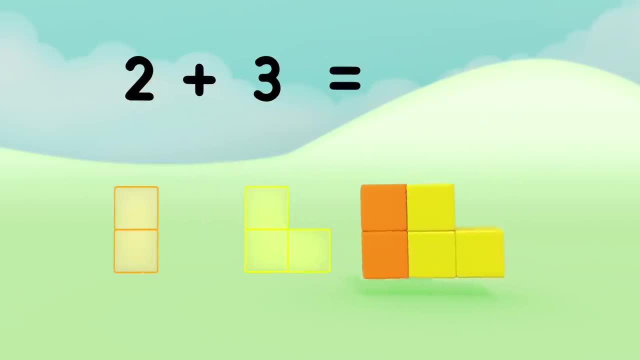 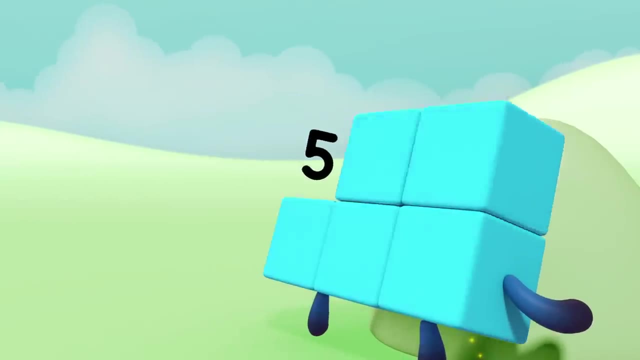 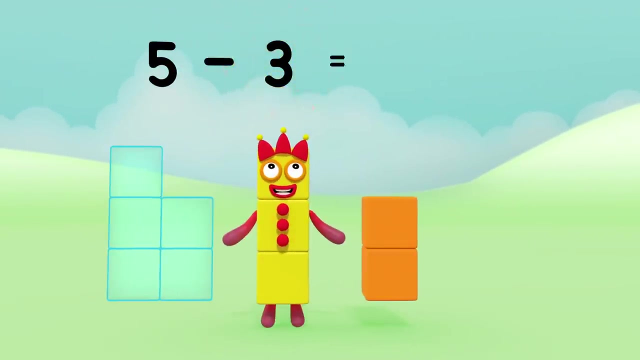 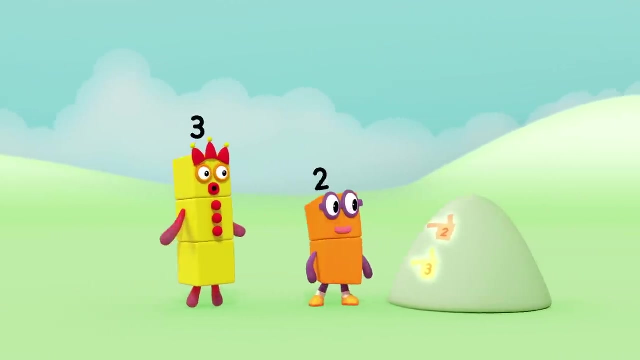 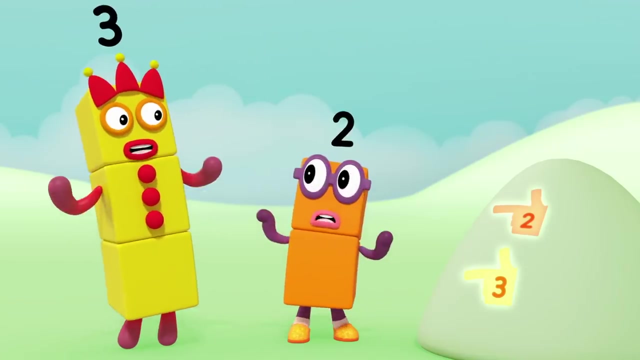 Two Plus three equals five Plus three equals five. Ready or not, here I be. Find you two, find you three. Five minus three Equals two. A pair of pointing prints, Five founders, But how, Eh Five. 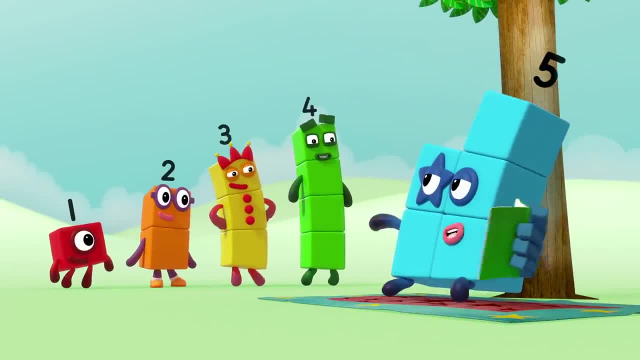 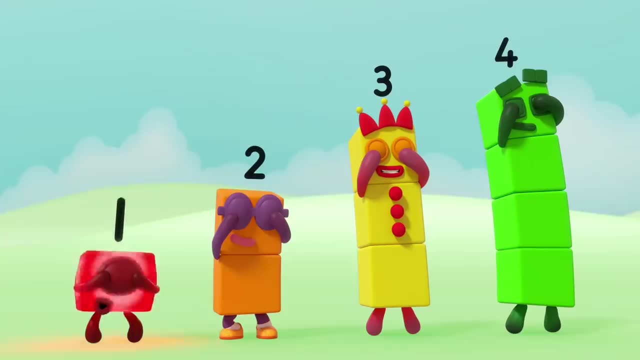 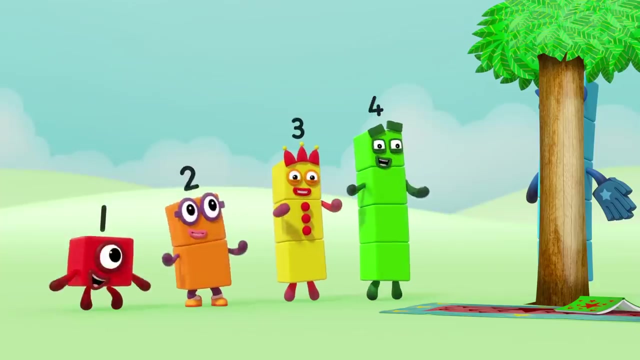 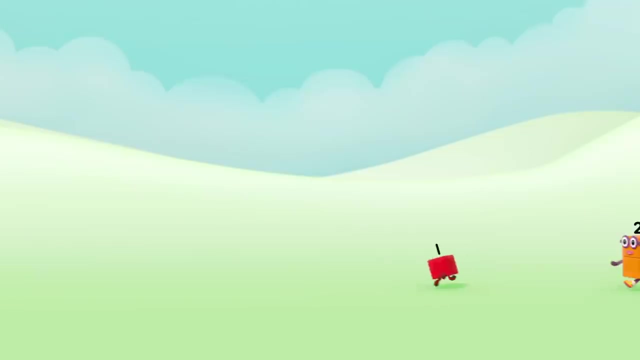 You're here. How did you Told you I was good. Now my turn to hide. We're done. One, two, three, four Ready or not? five, here we come, Ooh Rock. One plus four equals. 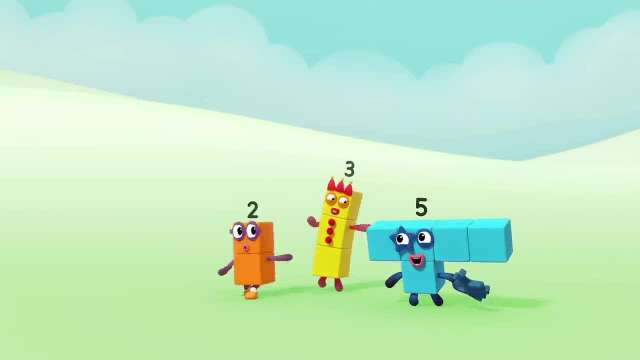 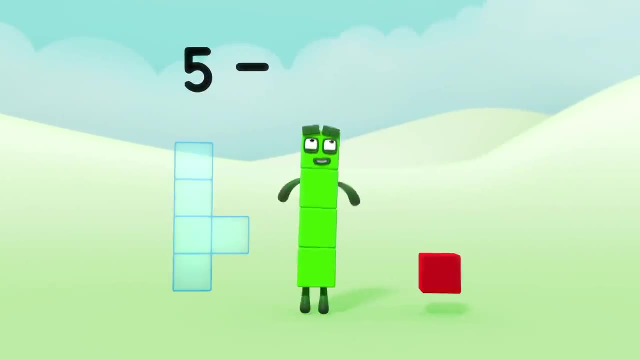 Five Found you, Amazing. Can you find me again? Five Minus four Equals one. Come on Rock. Three plus two equals Five. Found you Five? Fantastic. Can you find me again? Five Minus two. 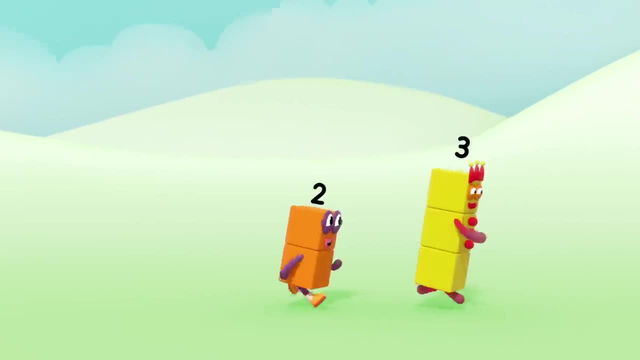 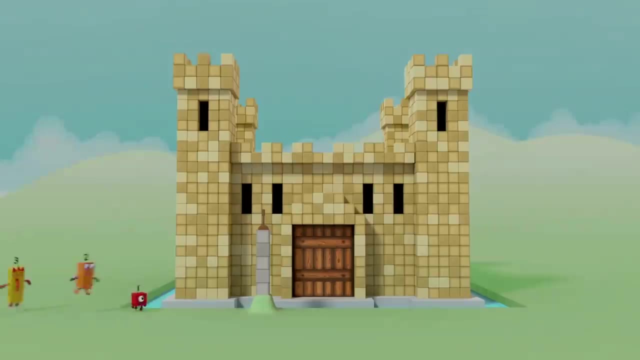 Equals three Found you. Ha ha ha. Five Minus two Equals three Found you. Ha ha ha, I found you. Ha ha ha, I found you. I found you. We found you, I found you, We found you. 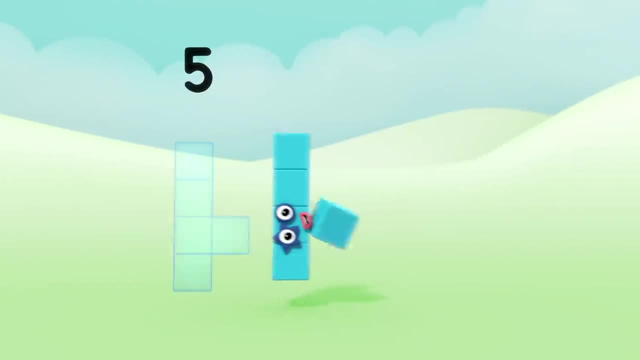 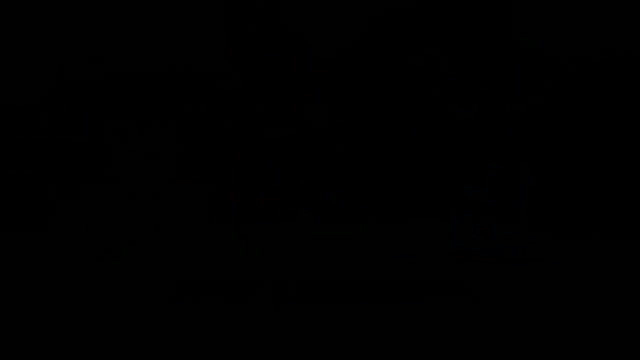 Can you find me again? Five, Five. Five minus four equals one. Come on, Rock. Three plus two equals five. Found you, Fantastic. Can you find me again? Five minus two equals three. Found you, Great. How do we get in? 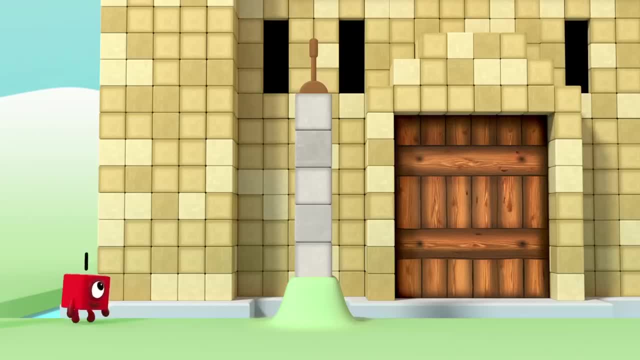 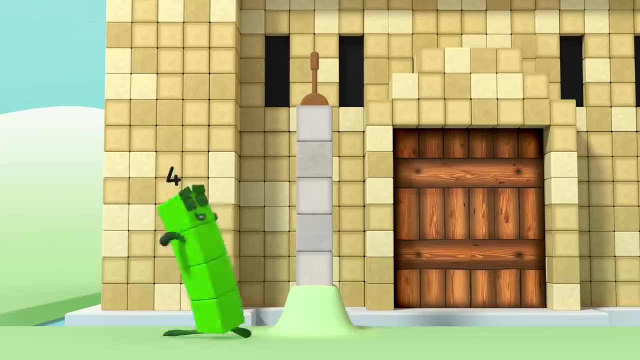 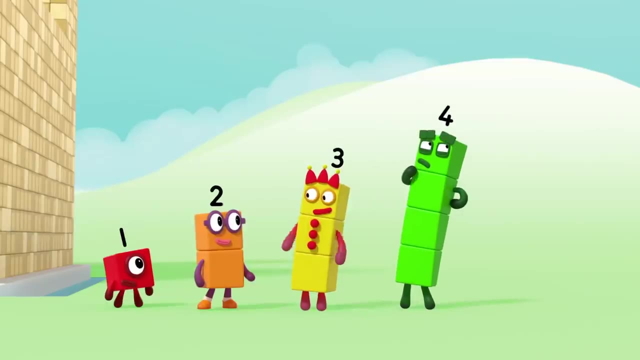 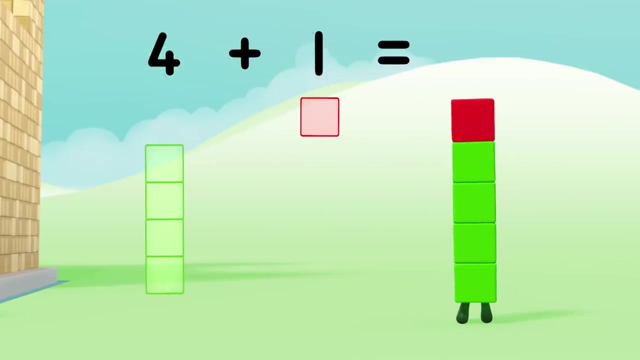 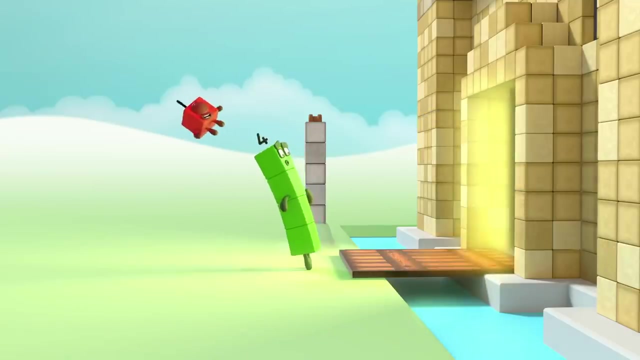 Maybe if we pull that handle. Oh, if only I was a little bit taller, Five's taller than four. So how do we get five? Four plus one equals five, Five, Woo-hoo, Woo-hoo, Woo-hoo. 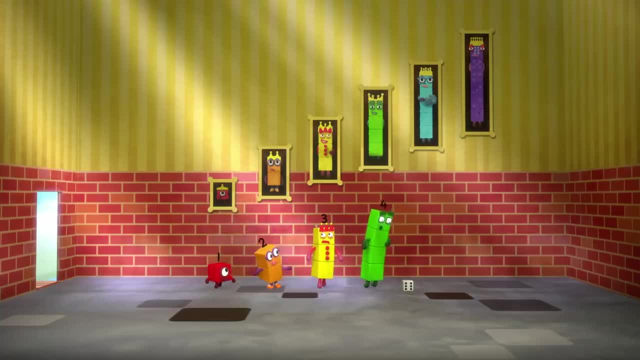 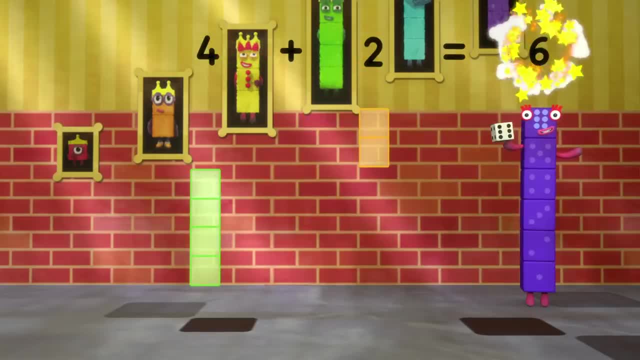 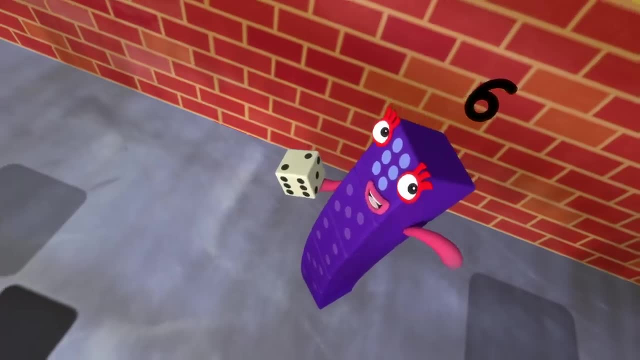 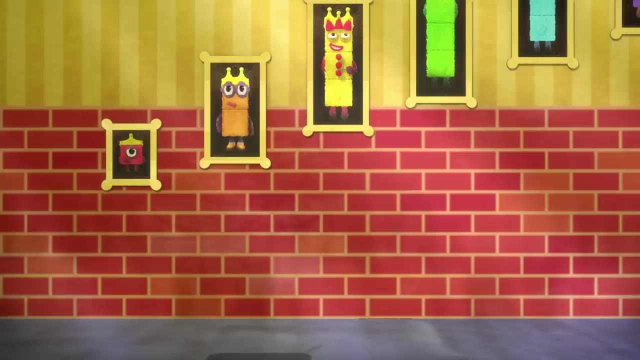 Four plus two equals six. Hello friends, Here's my advice. It's time for me to roll the dice. Watch me give a little throw and you'll know which way to go. One, two, three. Jake. One, two, three. 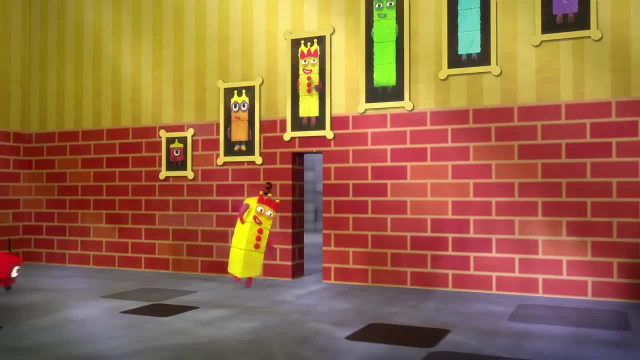 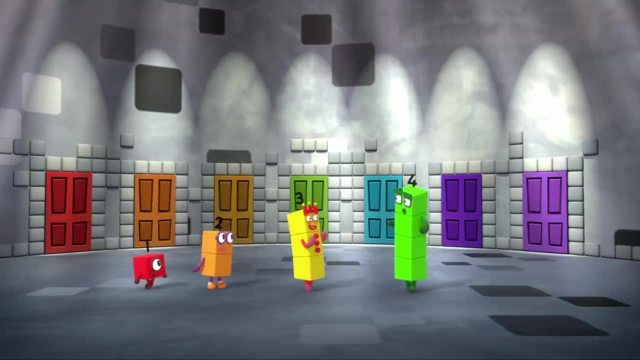 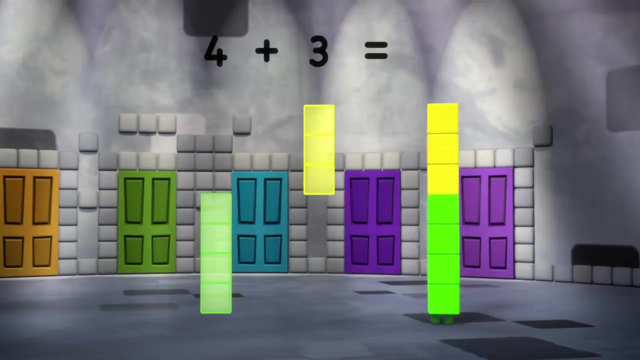 One, two, three. Follow me. Seven doors. Which door is right? Maybe seven can help. How do we get seven? How do we get seven? Four Plus three Equals Equals Seven. Oh, I fear you, Jake. 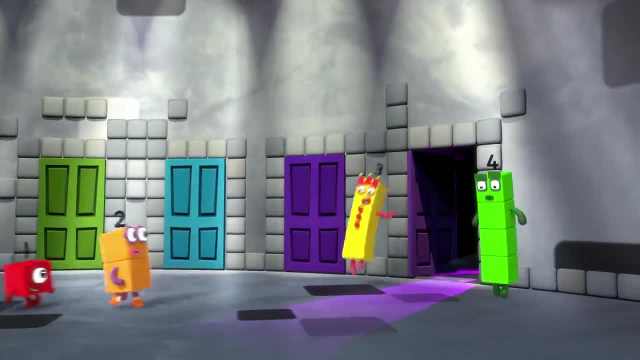 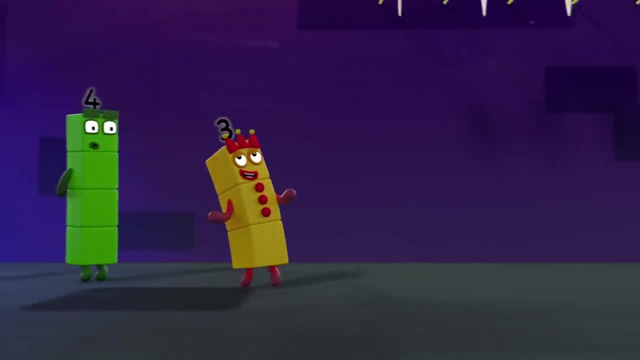 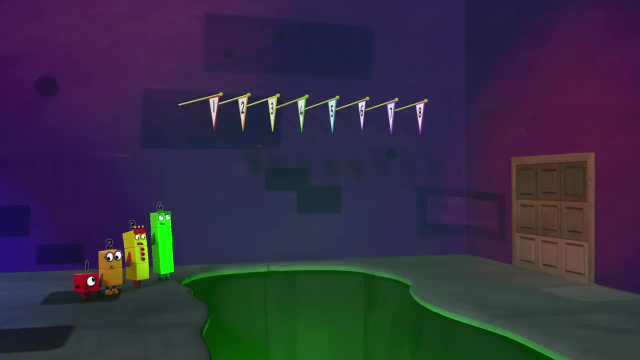 Oh, I fear you. I feel lucky This way, Easy peasy. Look at measy, We're stuck. No, we're not. We could swing from the flagpoles. We'd need someone with very long arms to stretch that high. 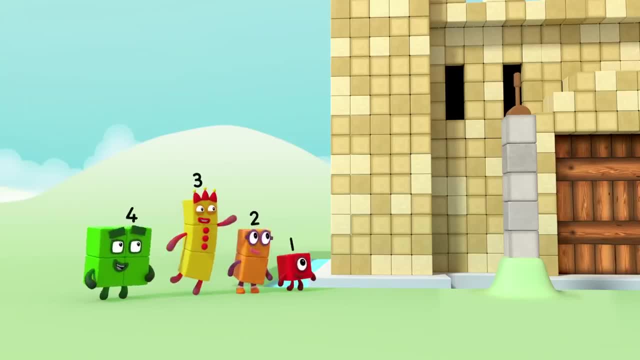 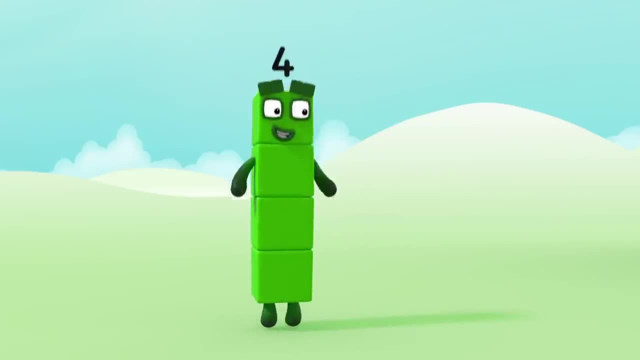 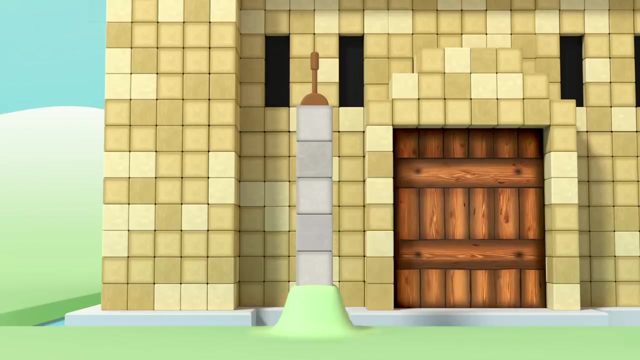 I see We found you, I see I saw you. Here we go, One Two, One, Two And one, And one. One, One, One, Three. Oh, I found you. Here you are. Here you are. 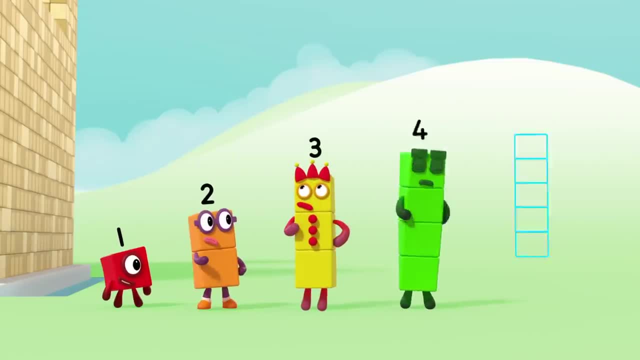 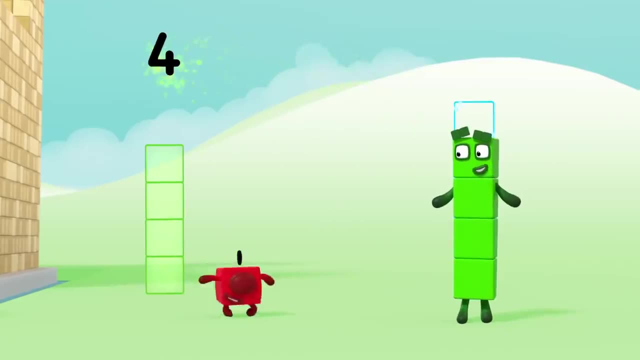 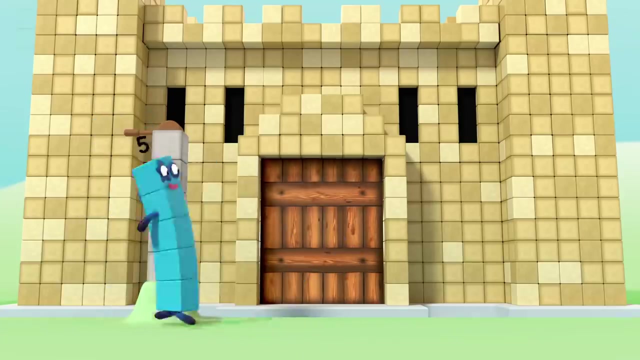 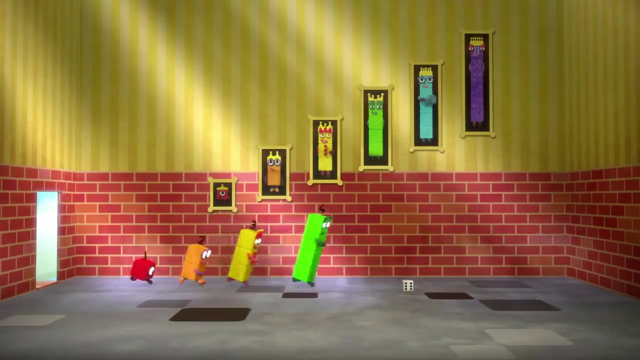 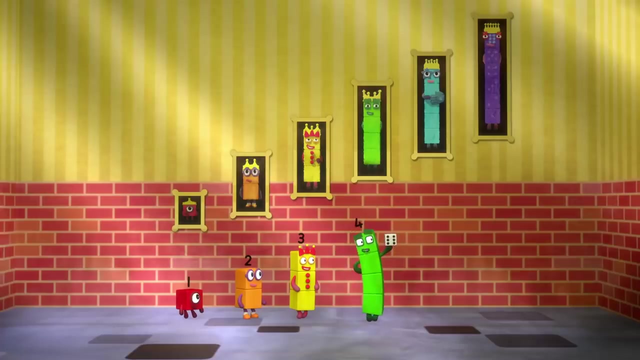 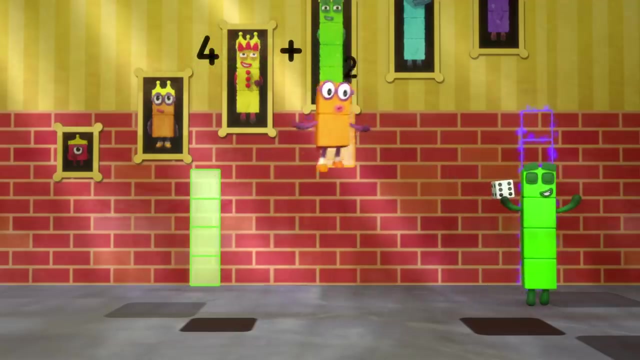 Five, One, Two, Four, Three, Four. Five. Four Plus one Equals Five. Dead end: Six is good with dice. How do we get six? Four plus two Equals Six. Hello friends, Here's my advice. 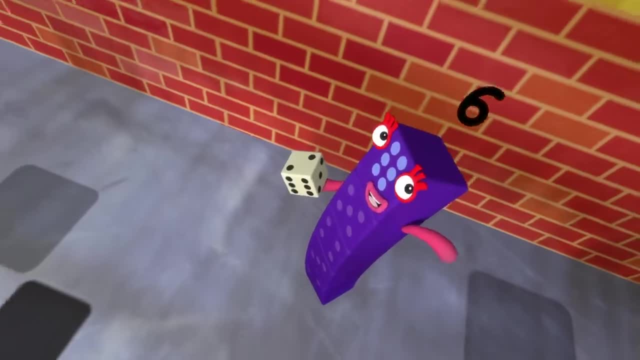 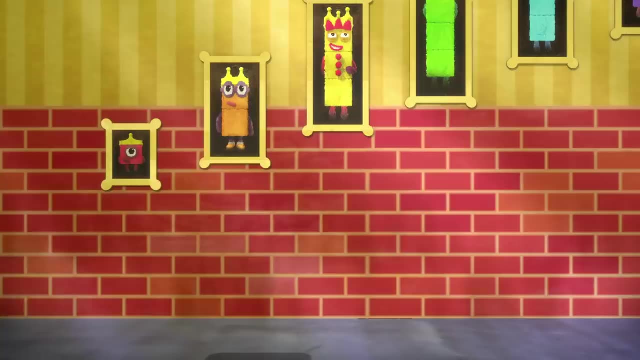 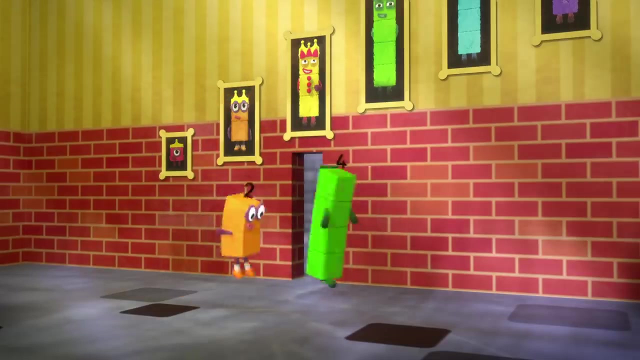 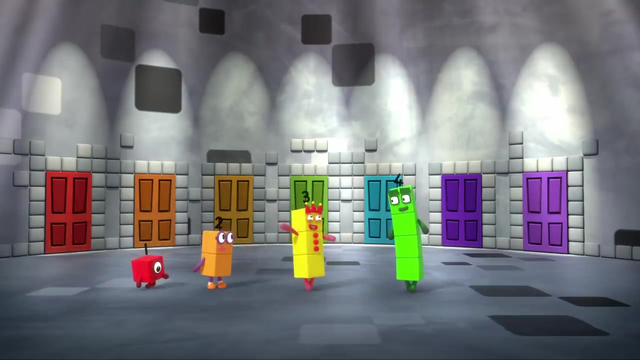 It's time for me to roll the dice. Watch me give a little throw and you'll know which way to go. One, two, three. One, two, three. Follow me. Seven doors. Which door is right? Maybe seven can help. 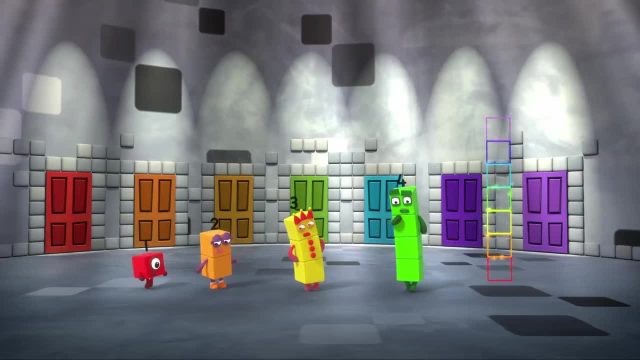 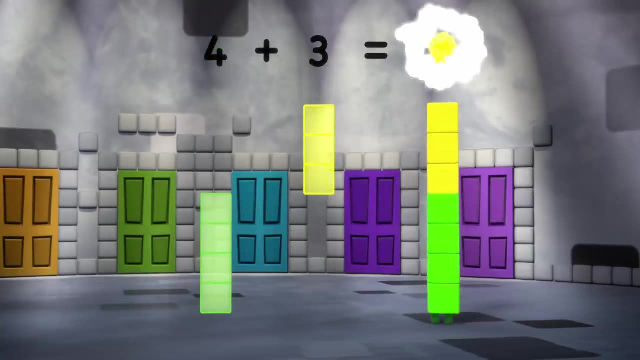 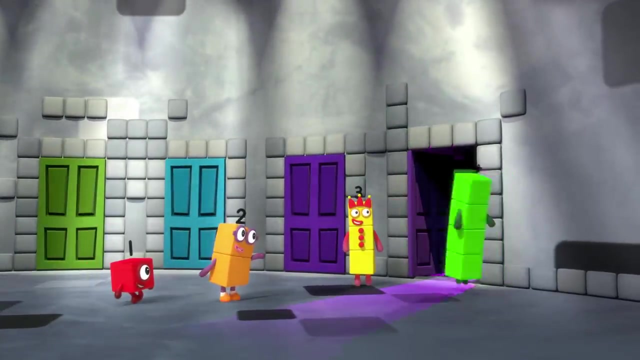 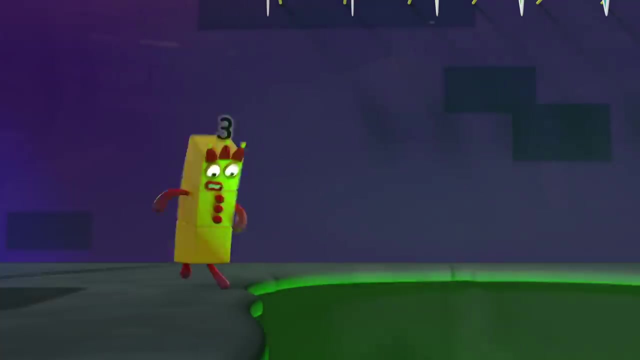 How do we get seven? Four Plus three Equals Seven. Oh, I feel lucky This way, Easy peasy. Look at measy, We're stuck. No, we're not. We could swing from the flag poles. 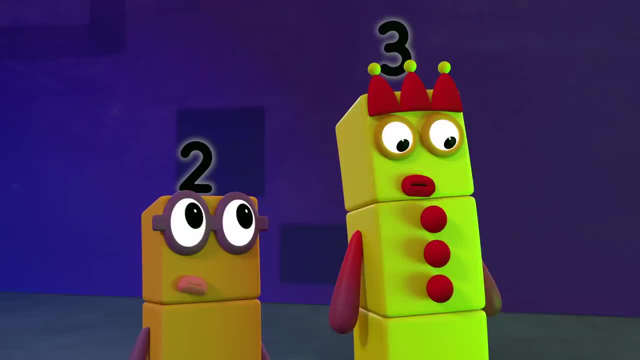 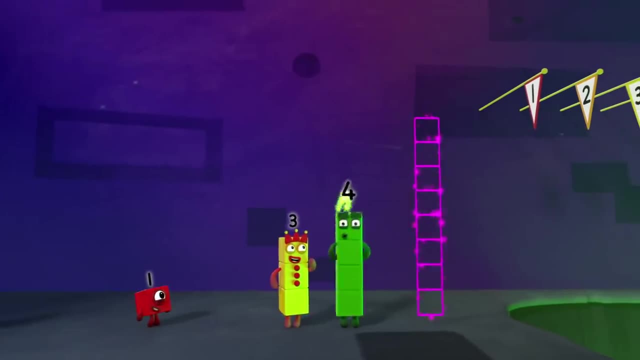 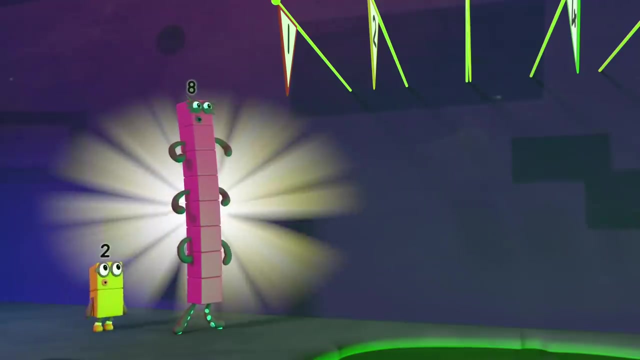 We'd need someone with very long arms to stretch that high. Eight: How do we get eight? Four Plus three Plus one Equals Eight. Octoblock swing: One, two, three, four, five, six, seven, eight. 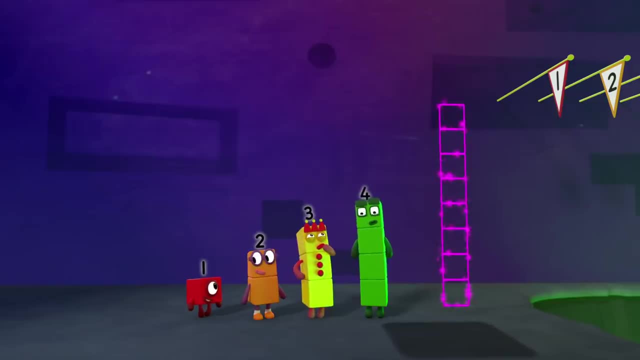 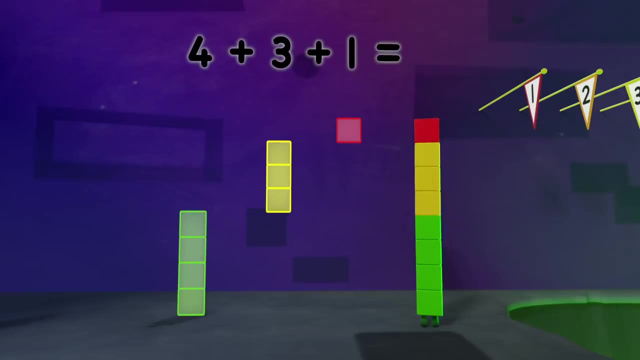 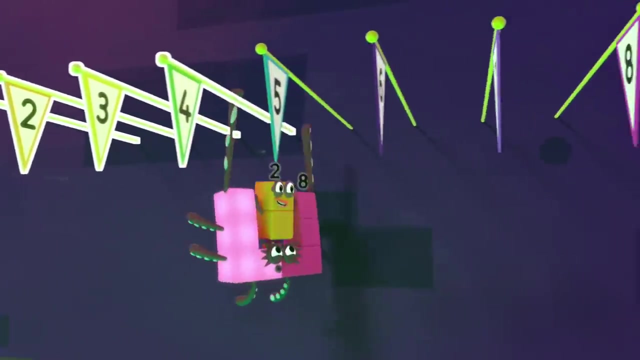 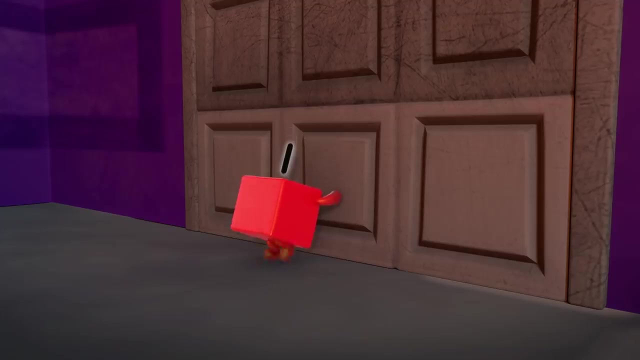 Eight. How do we get eight? Four Plus three Plus one Equals eight. Octoblock swing One, two, three, four, five, six, seven, eight. Swing It's stuck. Squares are strong. 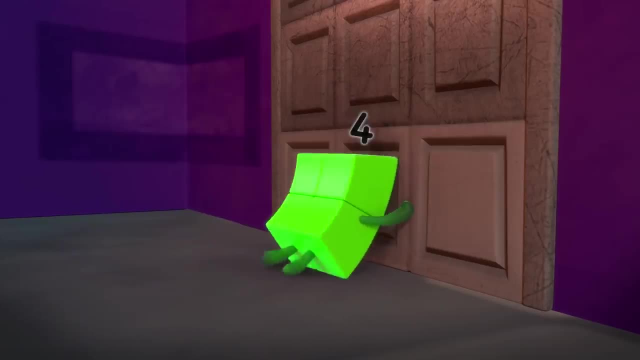 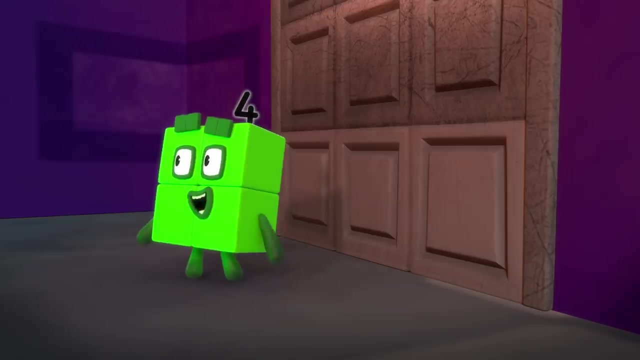 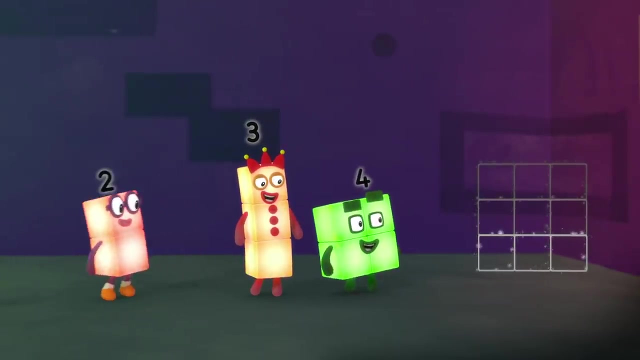 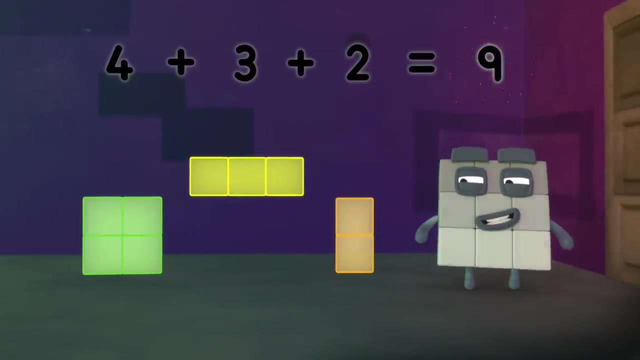 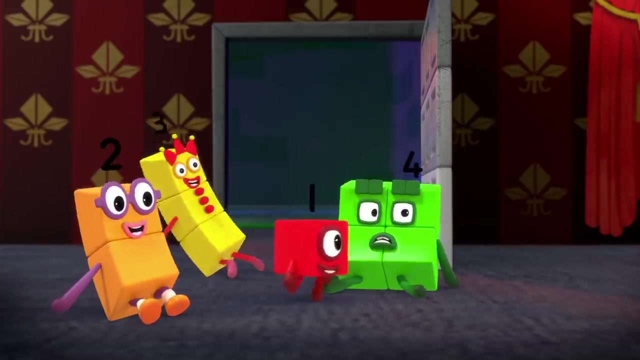 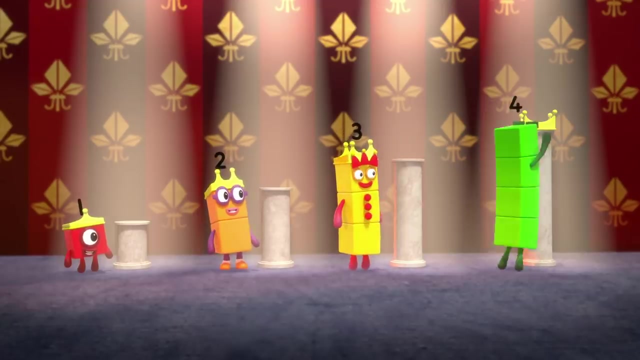 Let me try, Stop. We need a bigger square. Nine: How do we get nine? Four Plus three Plus two Equals nine. Thanks, Oh, One, Two, Three, Four, Four crowns, Cool, Uh-oh. 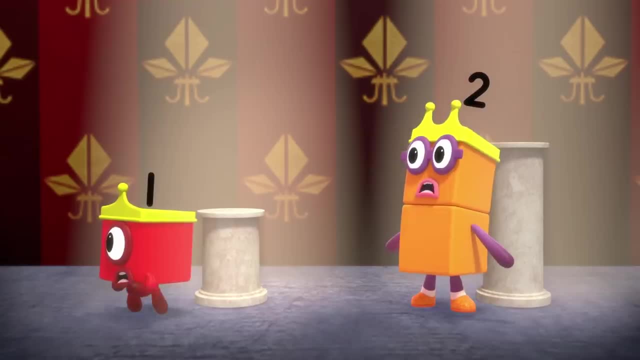 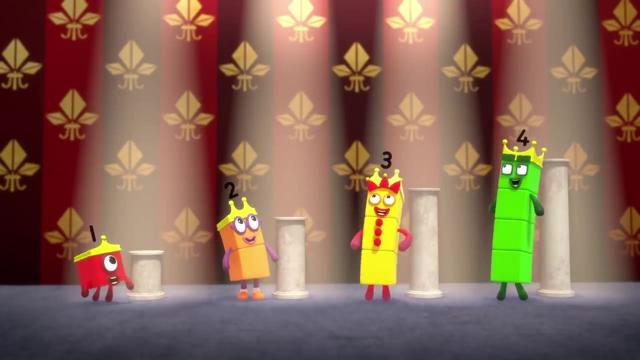 How are we gonna get out? If ten was here, we could rocket out through there. How do we make ten All together now? One, Two, Three, Four, Four Two. One, Two, One, Two, Three. 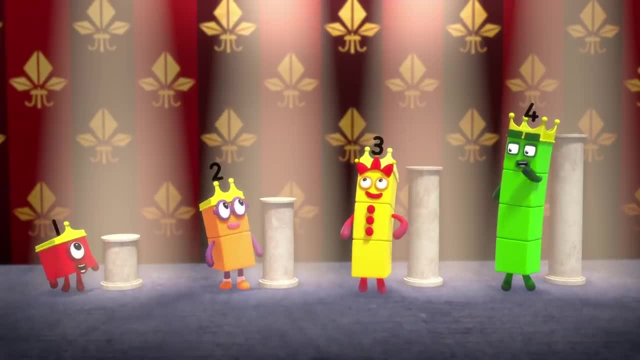 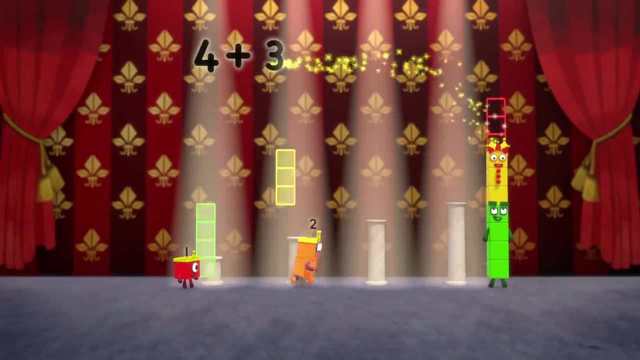 Four, Four, Two One Two, Three, Four Four Two One, Two, Three, Four Three, Two, Three, Two, Two One Two Two, One, Two, Four, Three, Two. 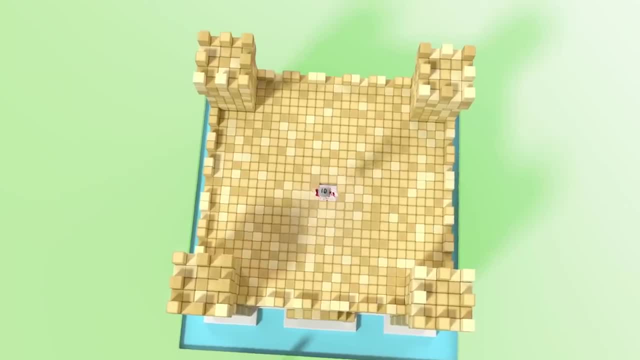 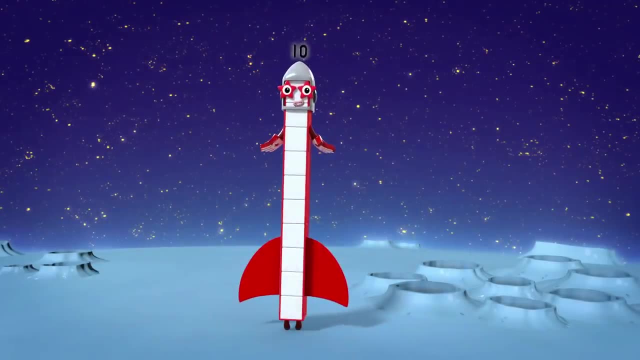 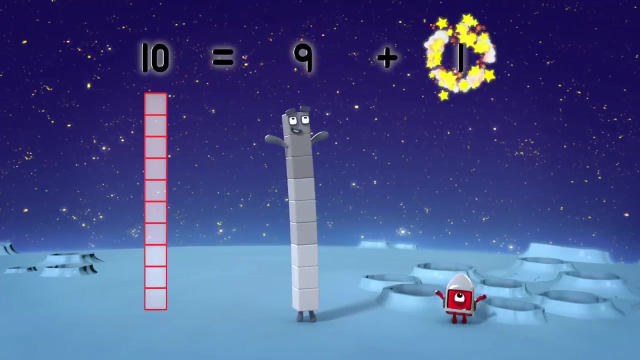 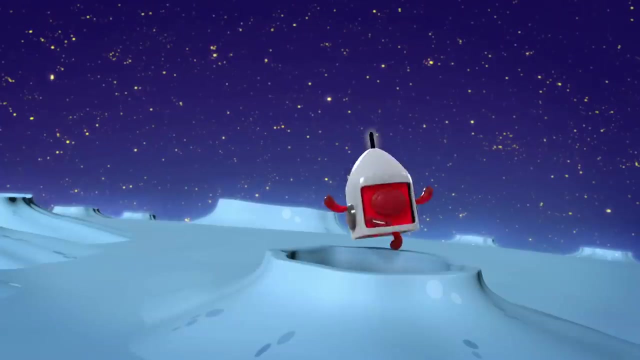 Three, Two, One, One, Ten, Ten, Nine, Eight, Seven, Six, Five, Four Friends will be here soon. Ten equals nine Plus one. One small step for a number, One giant hop for number kind. 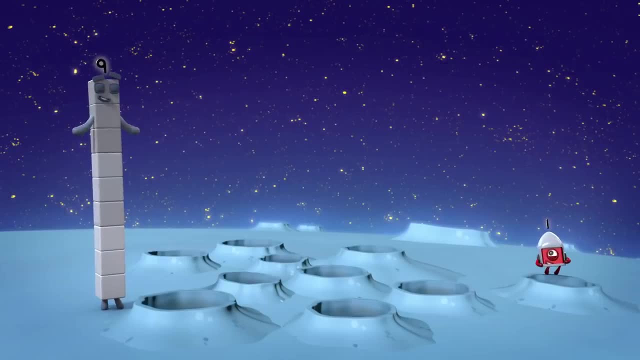 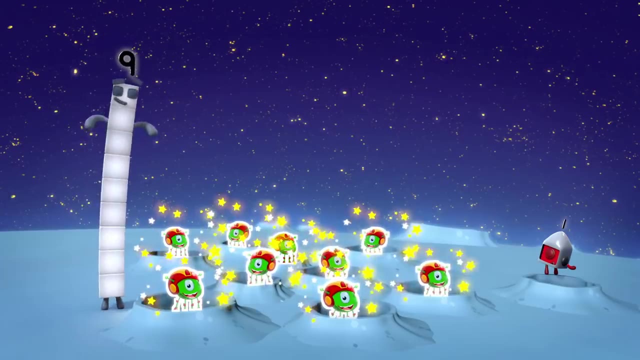 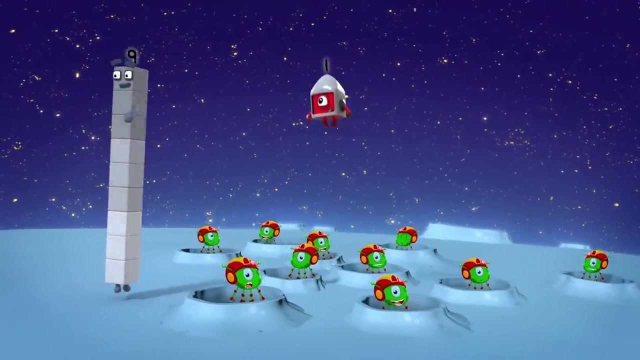 We're on the moon. Nine And one, That was easy, This is fun. One, two, three, four, five, six, seven, eight, nine, Nine aliens, And one more is ten. Wow, Nine plus one equals ten. 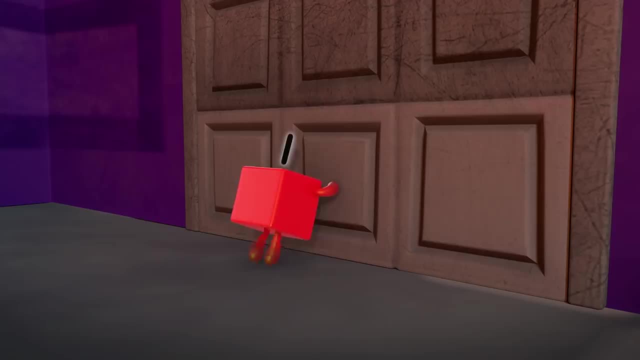 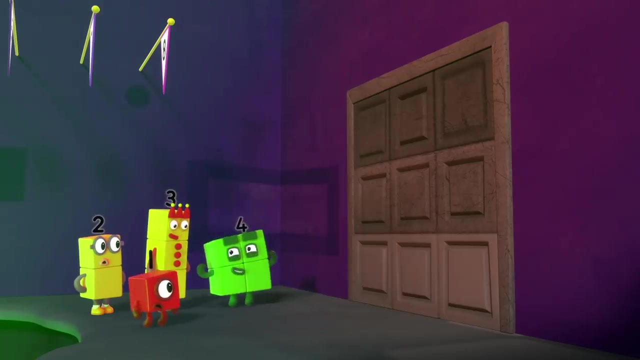 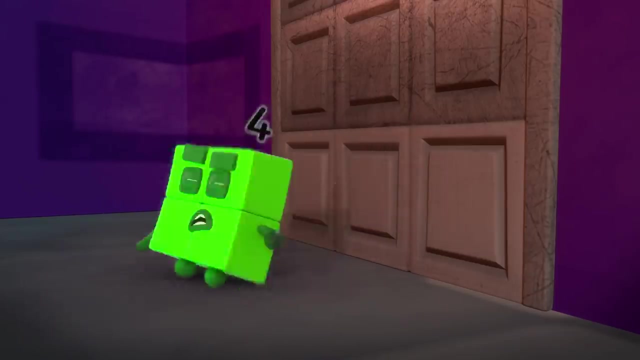 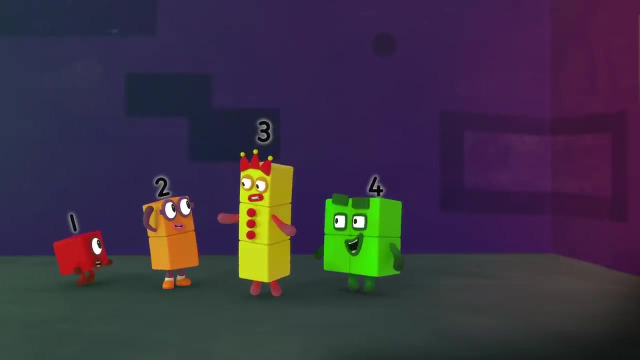 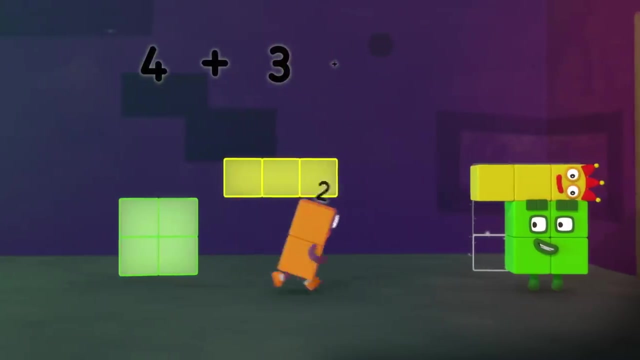 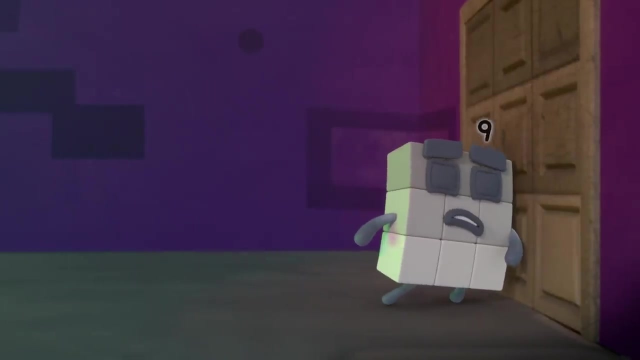 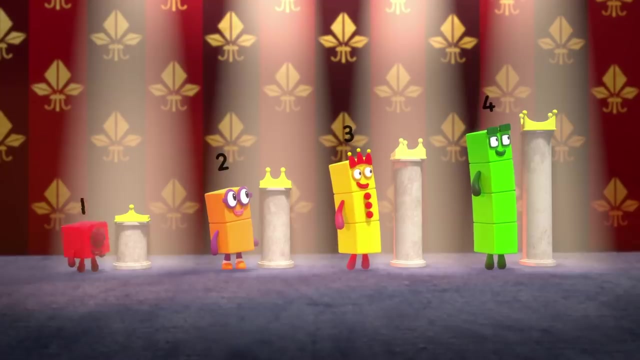 Swing- Yes, Fun, We made it And I won Six, Seven, Eight And nine Plus three plus two, equals nine. Thanks, One, two, three, four, Four crowns- Cool, Uh-oh, How are we going to get out? 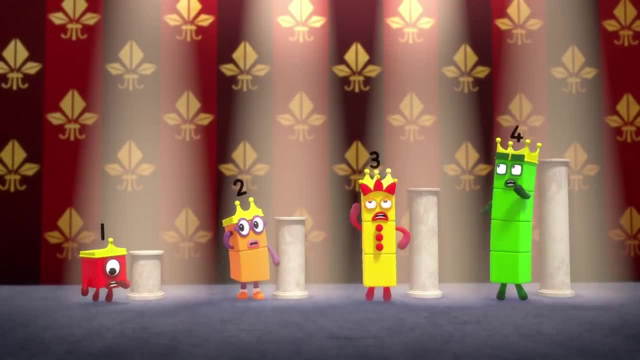 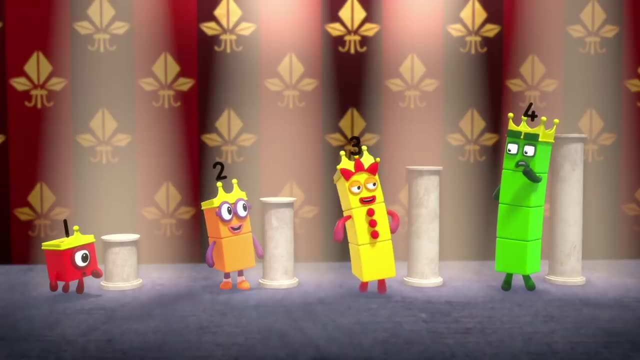 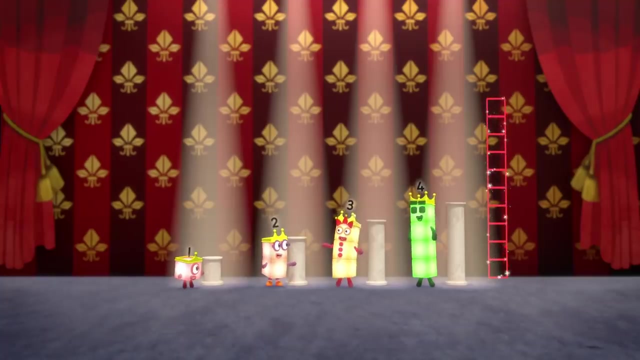 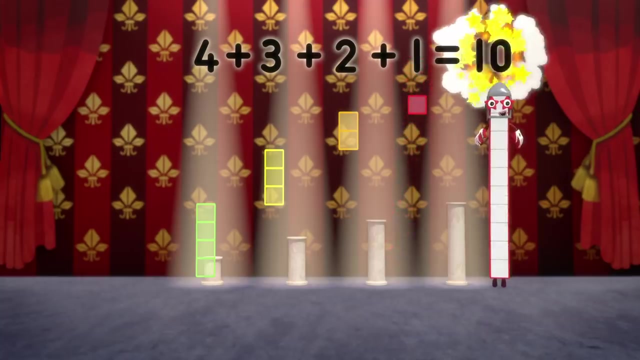 If ten was here, we could rocket out through there. How do we make ten All together now? Four plus three plus two plus one equals ten, Ten, nine, ten, nine, ten. Four plus three plus two plus one equals ten. 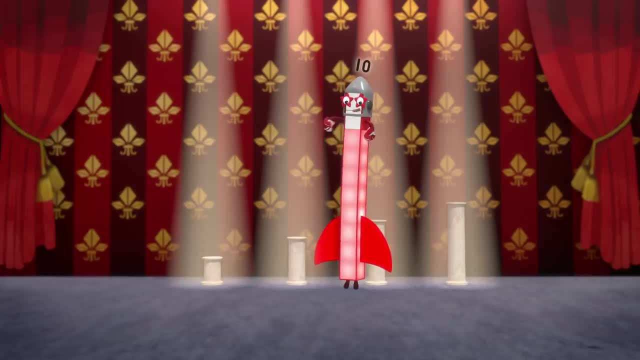 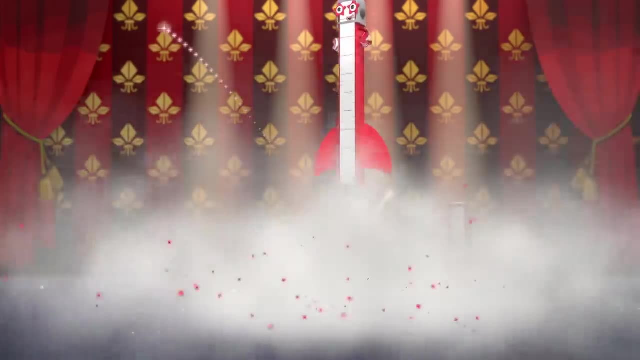 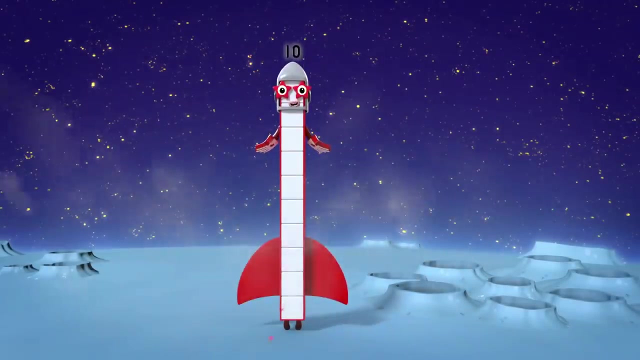 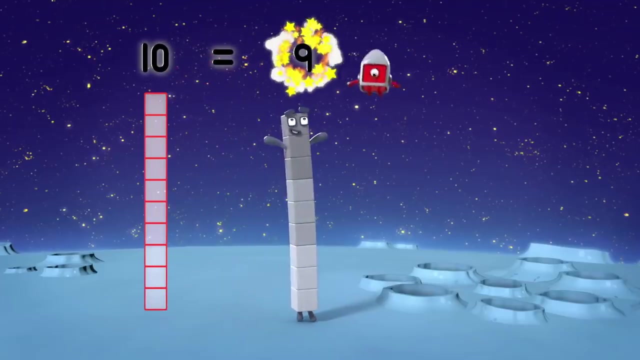 Ten, Ten, Ten, Eight, seven, six, five, four, three, two, one. Blast off Number ten up on the moon, And my friends will be here soon. Ten equals nine plus one. One small step for a number. 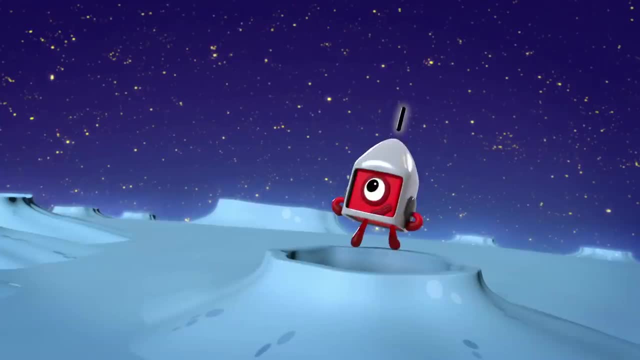 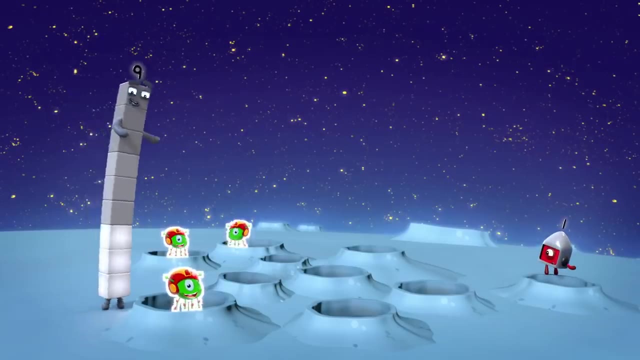 One giant hop for number kind, We're on the moon. Nine And one. That was easy, This is fun. One, two, three, four, five, six, seven, eight, nine, Nine aliens, And one more is ten. 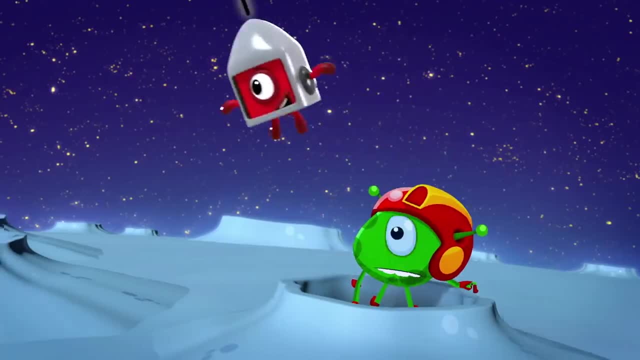 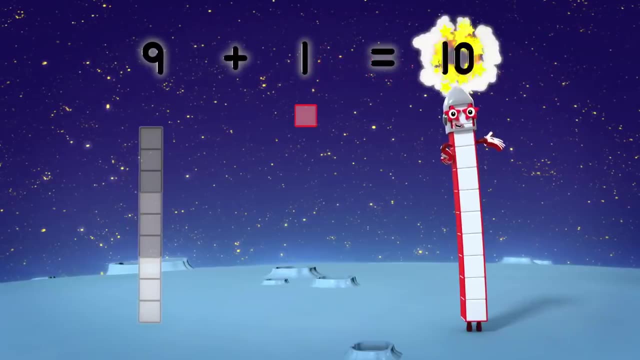 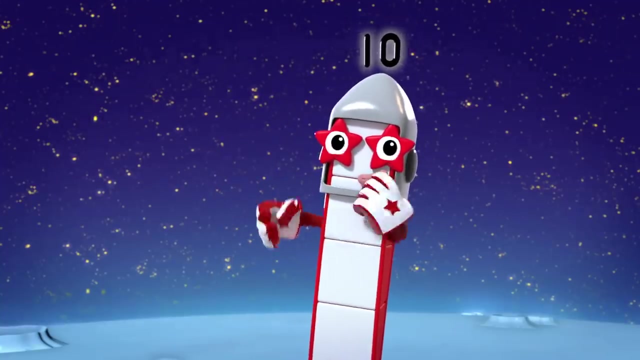 Whoa, Nine Plus one equals ten. Number ten back on the moon. Two more friends will be here soon. Nine, Nine, Nine And two. How did we get here? I haven't a clue. One, two, three, four, five, six, seven, eight. 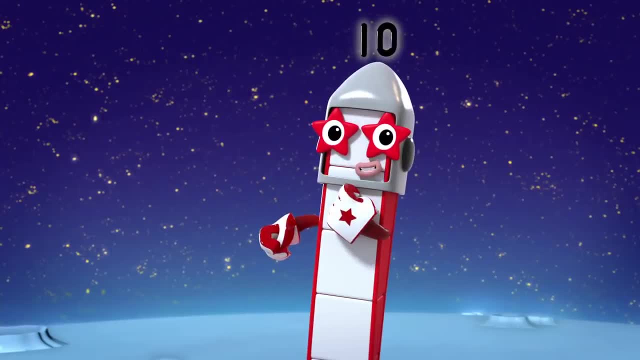 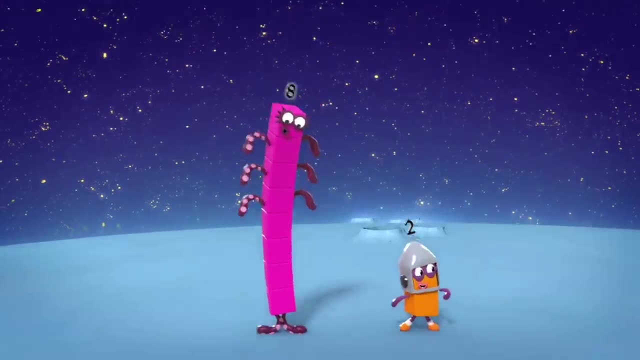 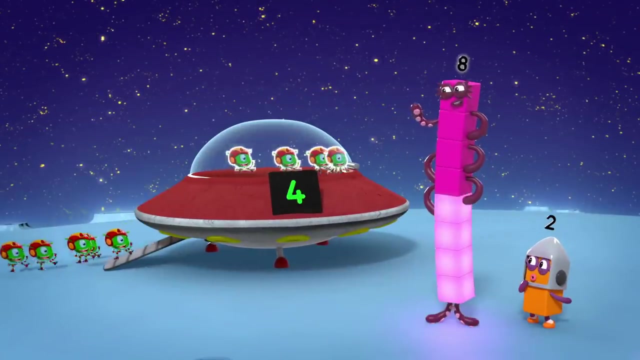 Number ten, back on the moon. Two more friends will be here soon. Ten equals eight plus two. We're on the moon. Eight And two. How did we get here? Haven't a clue? One, two, three, four, five, six, seven, eight. 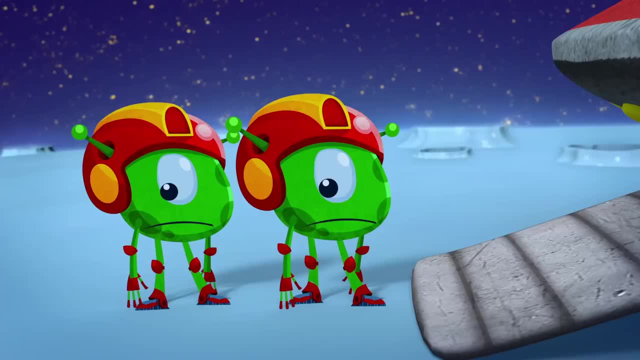 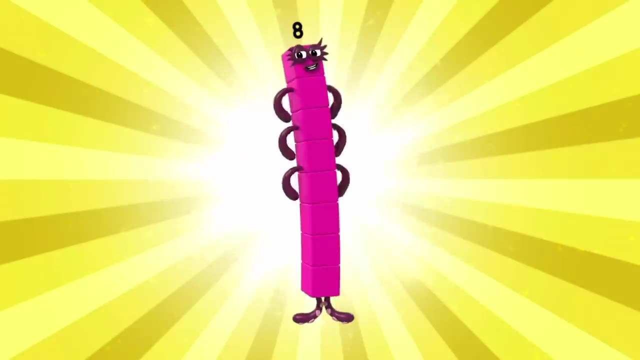 Eight aliens, All heads, And we're heading home. Oh no, There's no room for those two, Never fear. Octoblock is here. Octoblock Bill One, two, three, four, five, six, seven, eight. 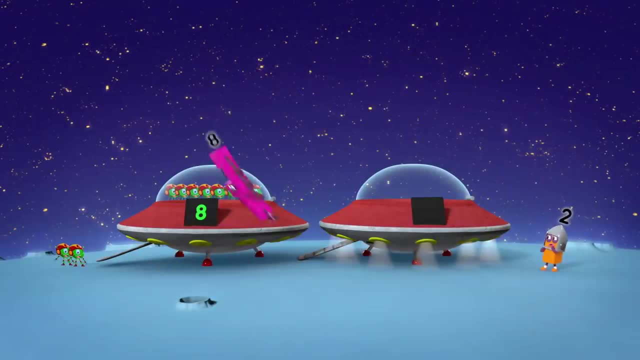 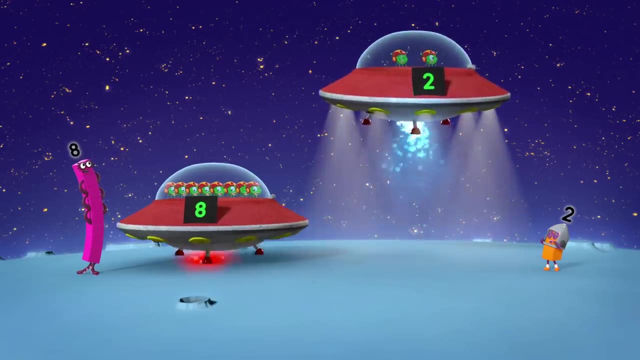 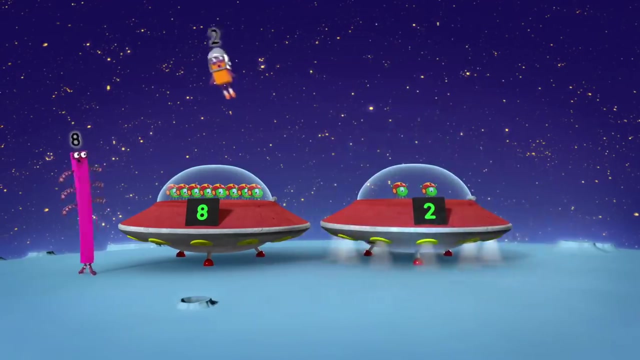 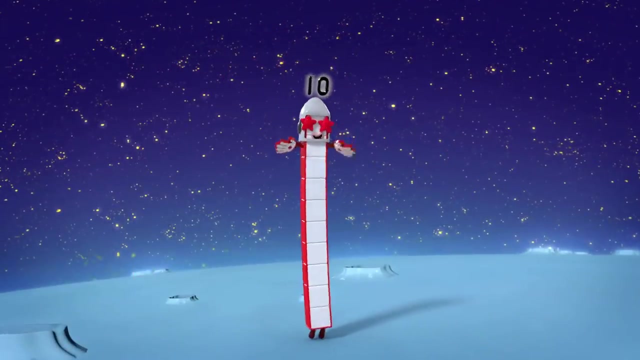 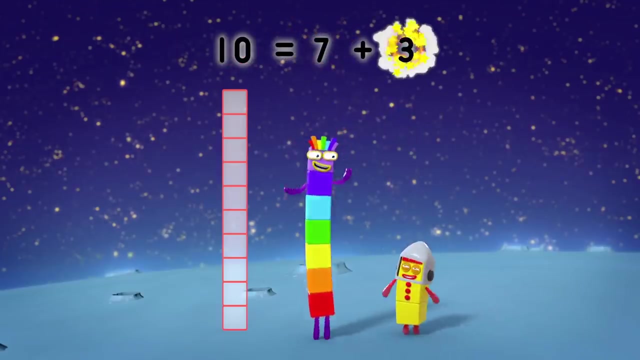 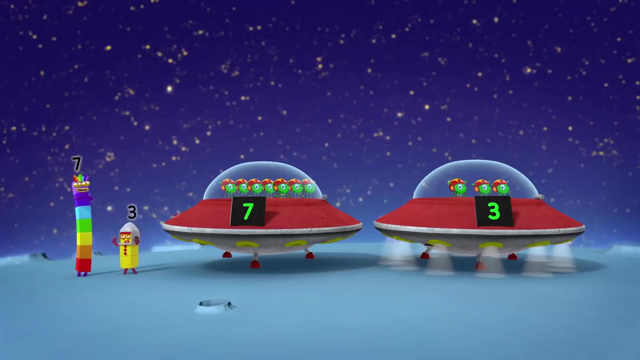 Bill Two: flying saucers. Good work. Aah, Aah, Aah. Oh, come back. It's not starting Time to make some friends again. ten equals seven plus three, Seven and three. we're so lucky There's the on button. 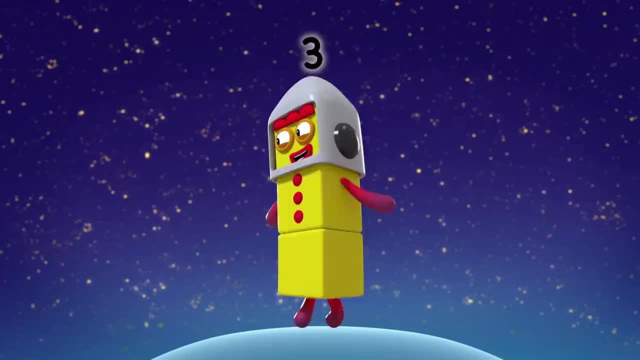 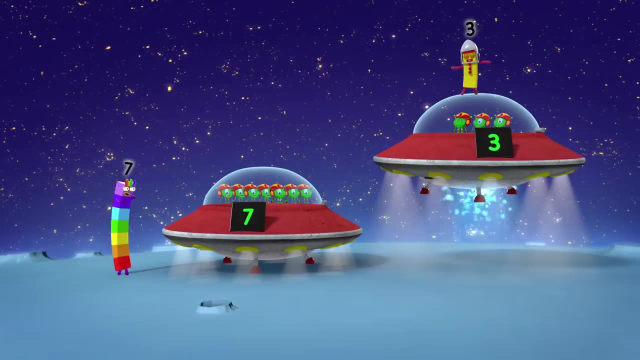 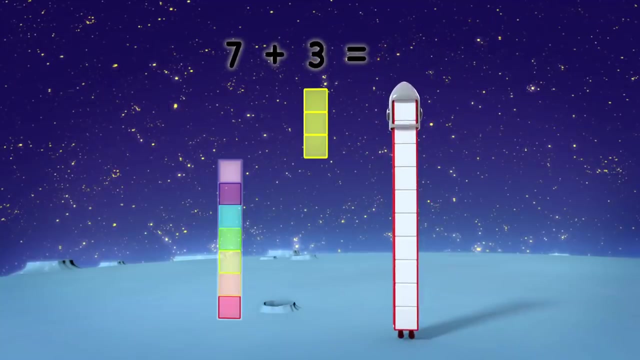 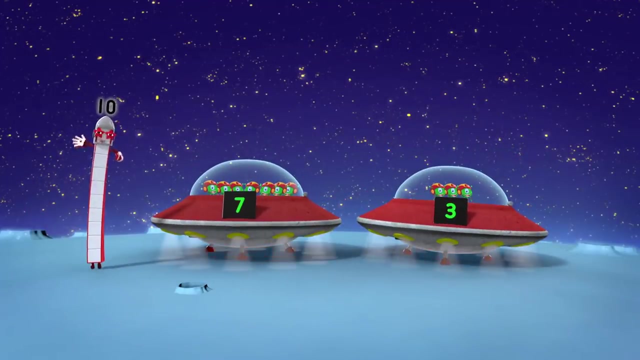 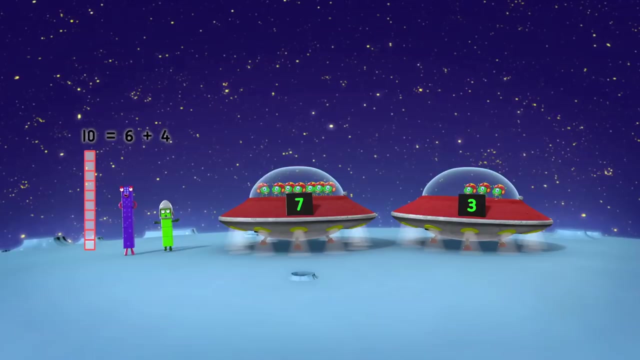 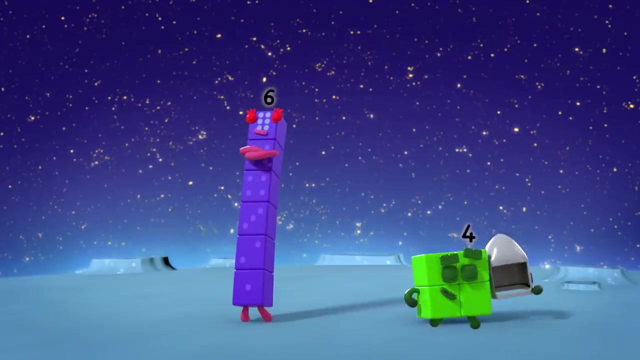 That was lucky, Ready, steady, blast off, It's too heavy. Plus three equals It's time again. wait and see who my next two friends will be. ten equals four. We're on the moon. six and four. we really couldn't ask for more. let's play a game: rule the dice and 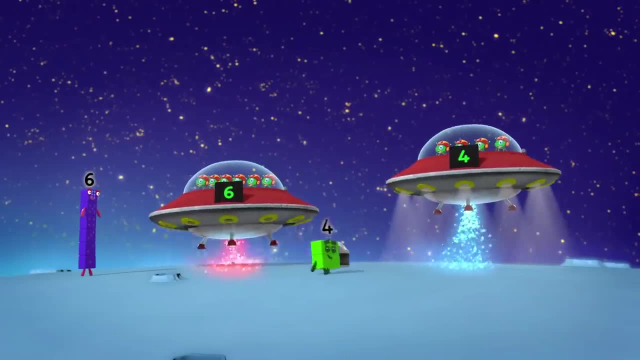 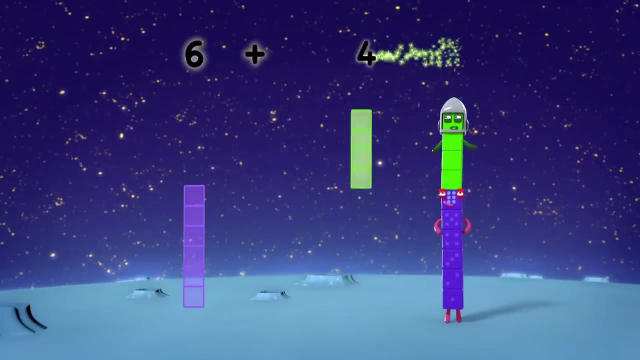 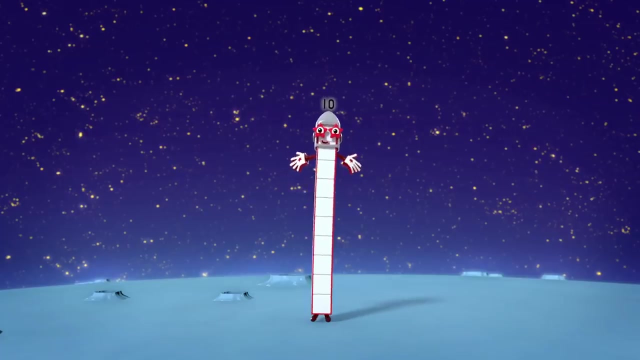 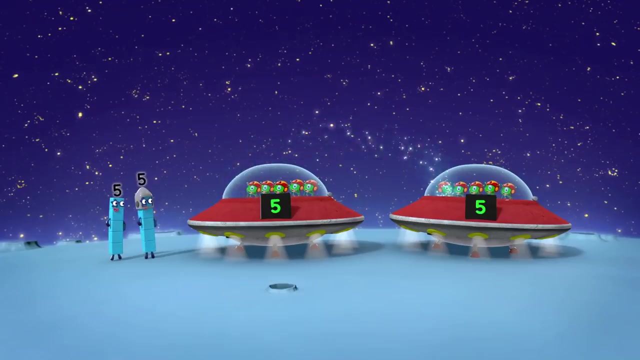 That was so cool, Still too heavy. Six plus four equals ten. Six plus four equals ten. Quick, before our visit ends, we've just got time for two more friends. ten equals five plus five. We're on the moon. five and five. it sure feels great to be alive. let's give them a hand. 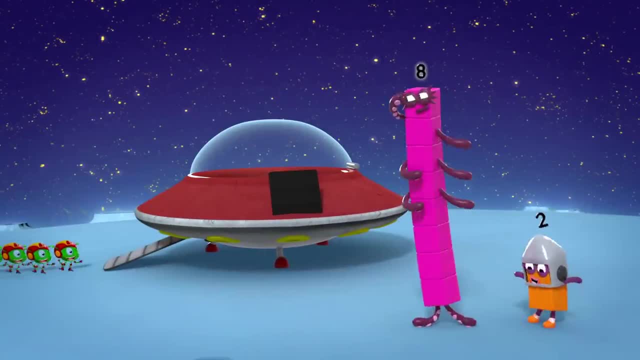 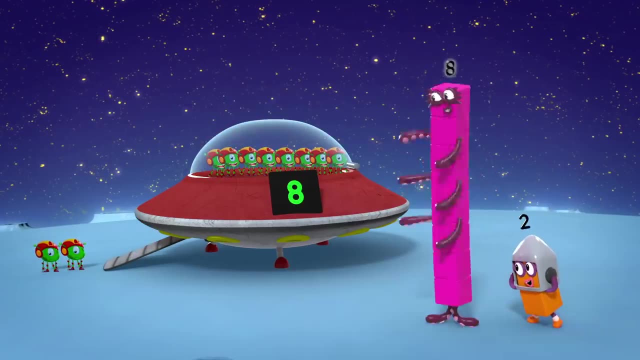 Eight aliens All heading home. Oh no, There's no room for those two, Never fear, Octoblock is here. Octoblock Bill One, two, three, four, five, six, seven, eight, Eight aliens. 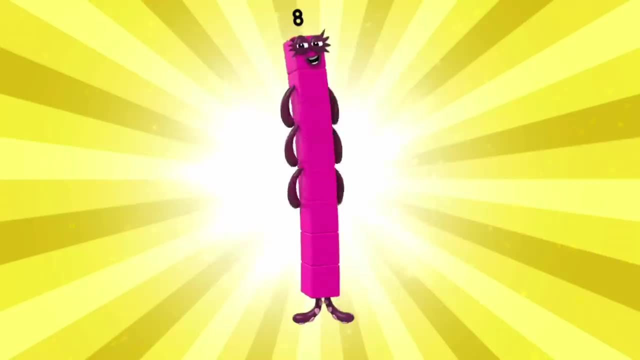 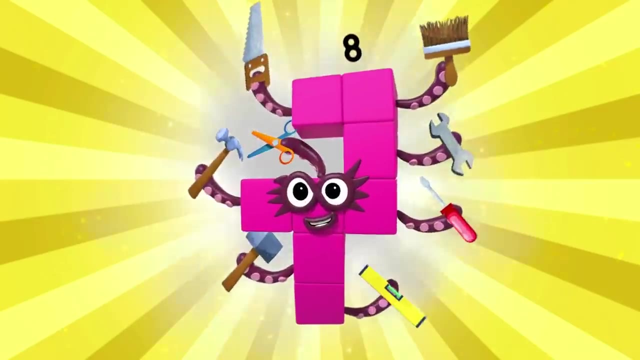 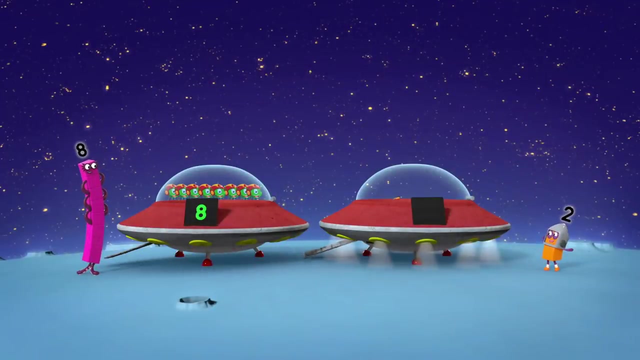 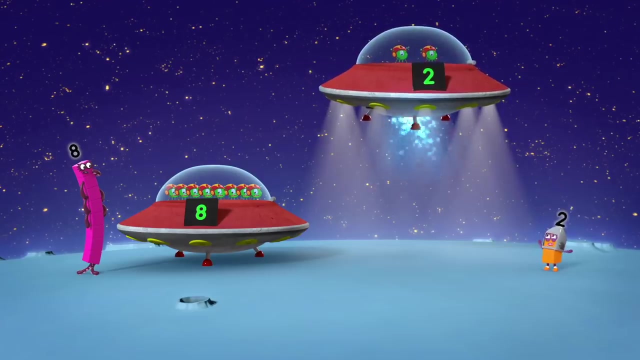 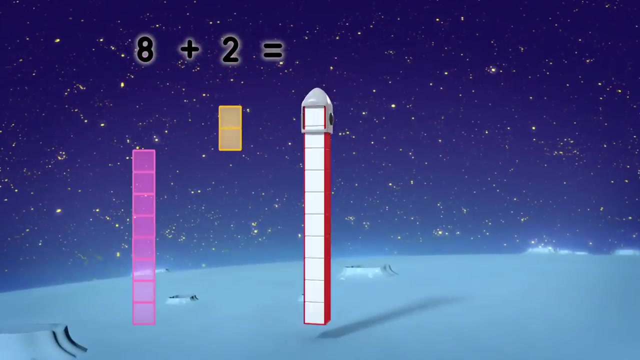 All heading home. One, two, three, four, five, six, seven, eight. One, two, three, four, five, six, seven, eight Filled Two flying saucers. Good work, Come back. It's not starting. Eight plus two equals ten. 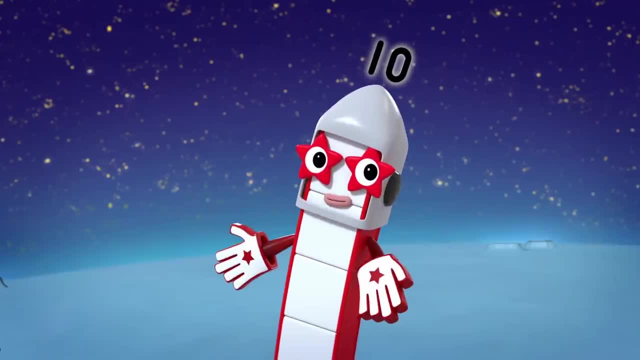 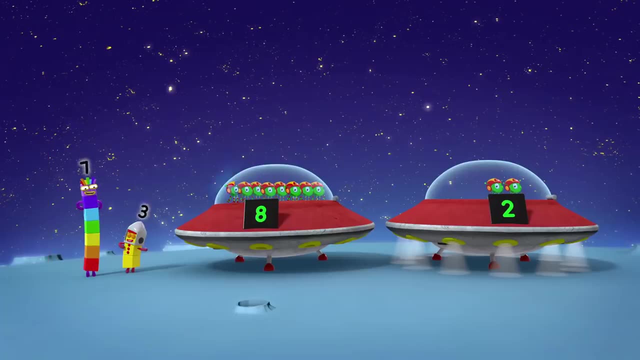 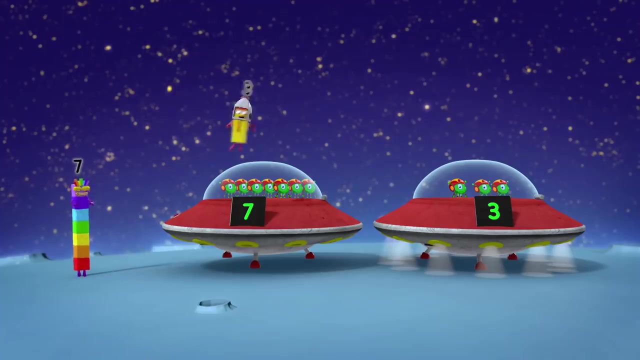 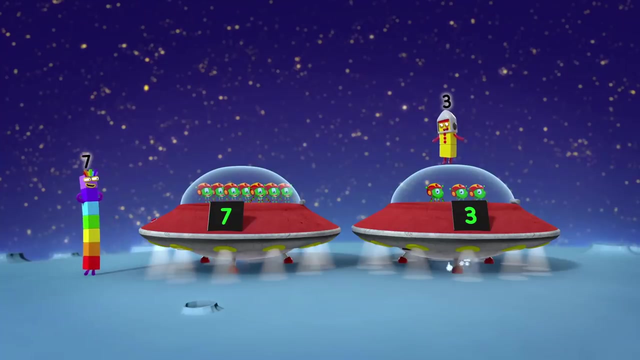 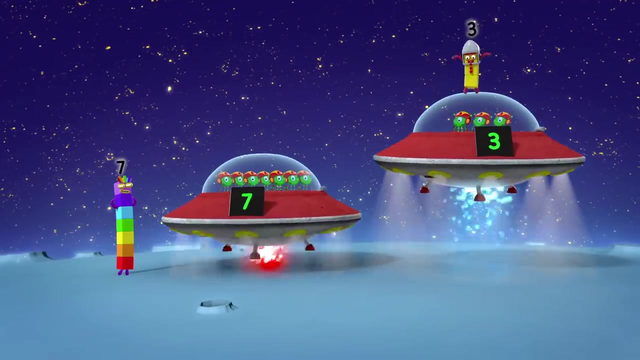 Here I am. number ten Time to make some friends again. Ten equals seven plus three. We're on the moon. Seven and three, We're so lucky. Look at me, Look at that. There's the on button. That was lucky, Ready, steady, blast off, It's too heavy. 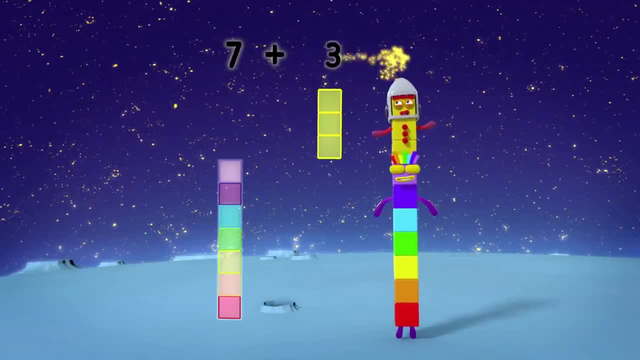 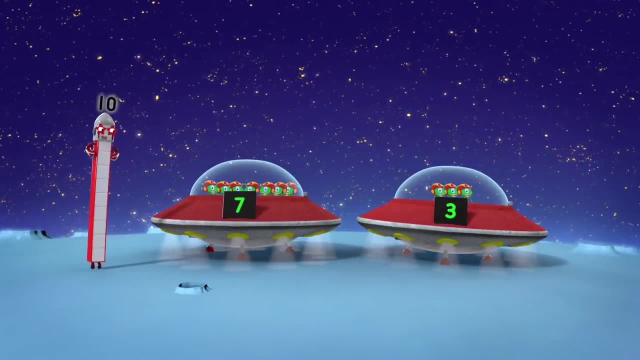 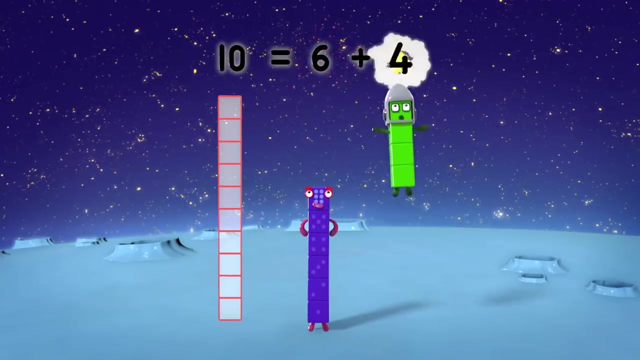 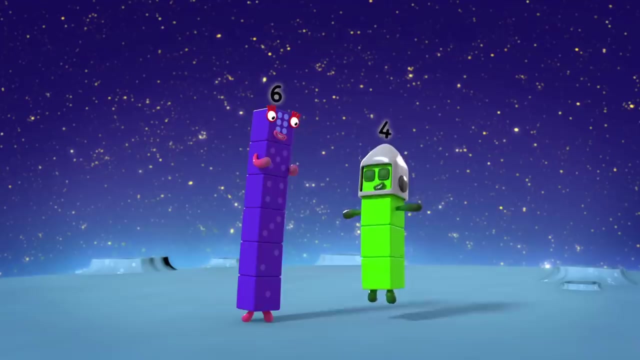 Seven plus three equals ten. It's ten again. Wait and see who my next two friends will be. Ten equals six plus four. We're on the moon. Six and four. We really couldn't ask for more. Let's go, Let's play a game, Roll the dice and 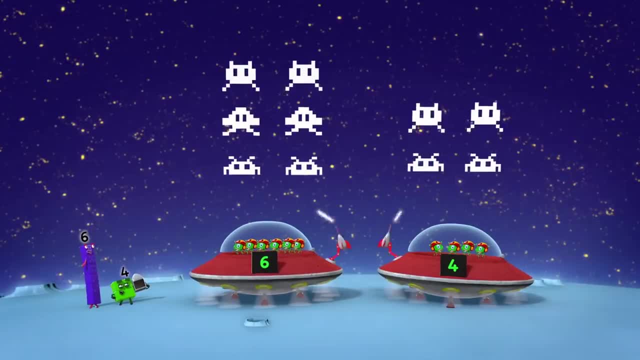 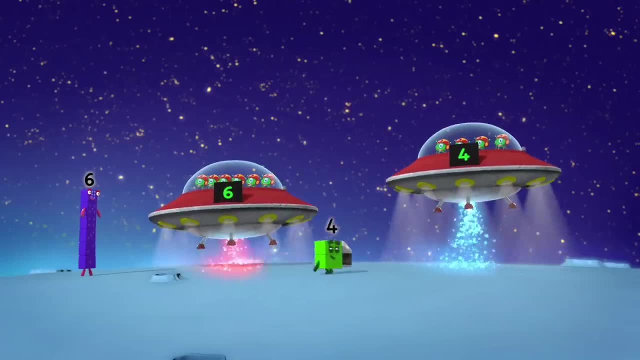 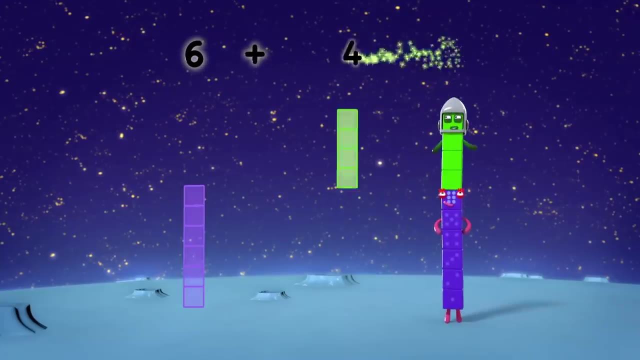 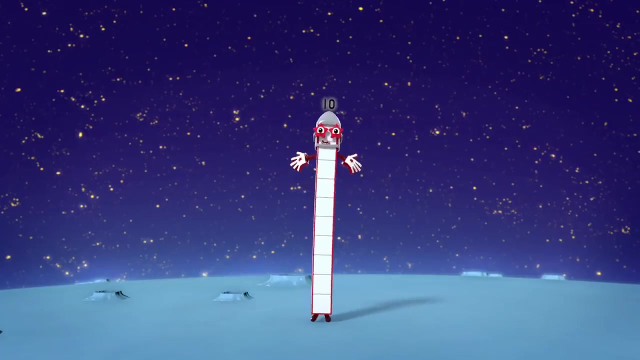 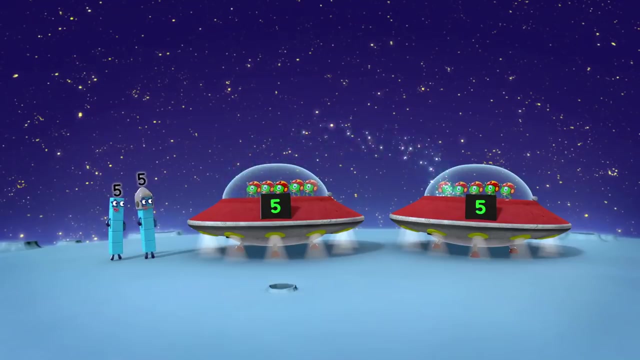 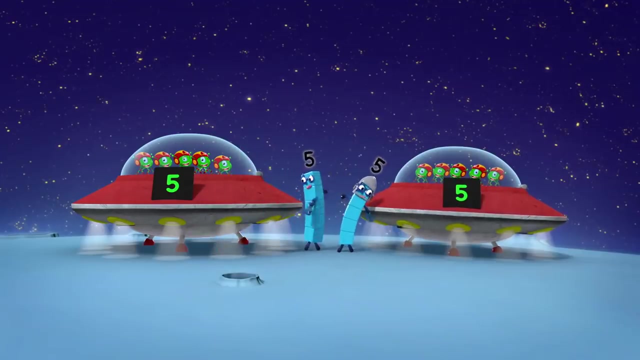 That was so cool. Still too heavy. Six plus four equals ten. Quick, before our visit ends, We've just got time for two more friends. Ten equals five. We're on the moon. Five and five. It sure feels great to be alive. Let's give them a hand, High five.